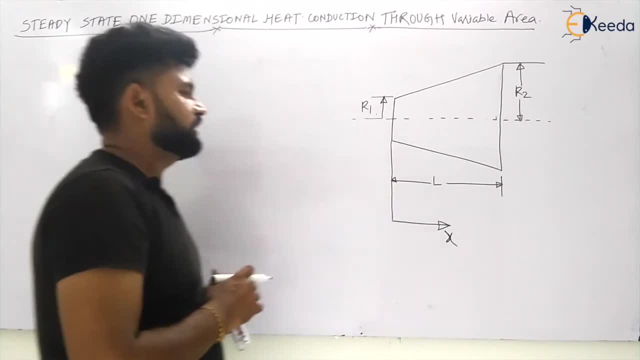 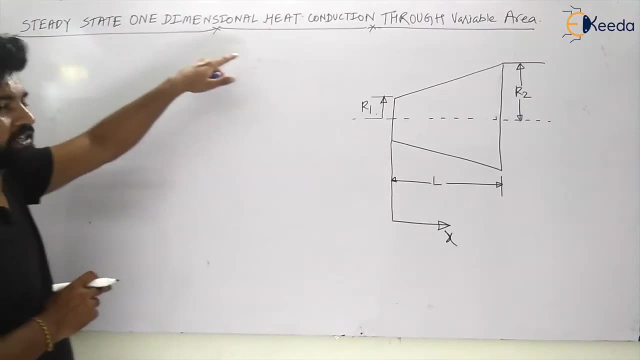 from R1 to R2, now in the x direction. you can see now. so if there will be heat transfer, so first of all we have assumed that there is a steady state, one dimensional heat transfer. so heat will be conducted through this, only this direction, that is, in x direction. that 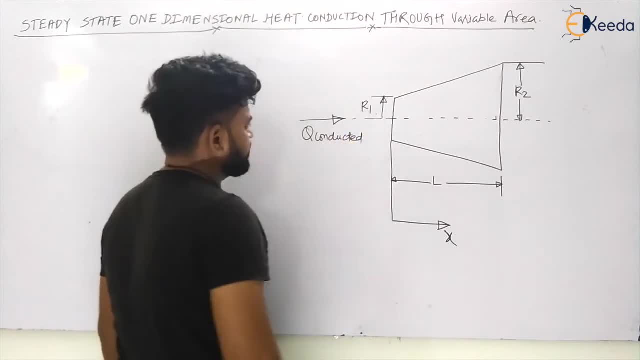 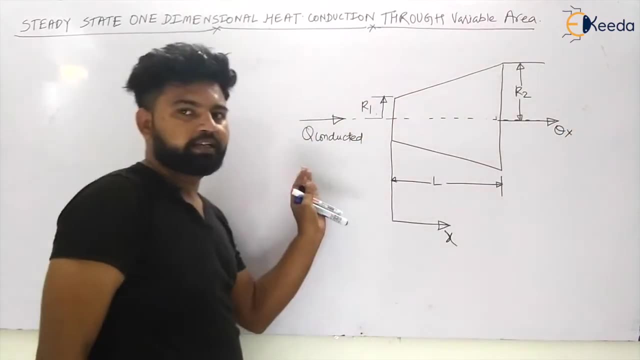 is Q conducted, it will be conducted through this direction and will be passed through this direction. so there will not be any heat transfer. there will not be any heat transfer from the x or y- sorry, y or z direction. so what I will do is I will just insulate. 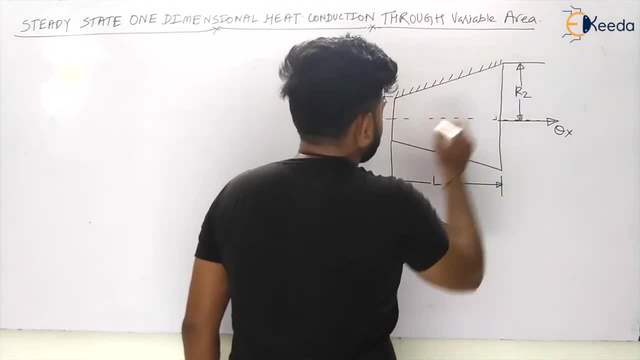 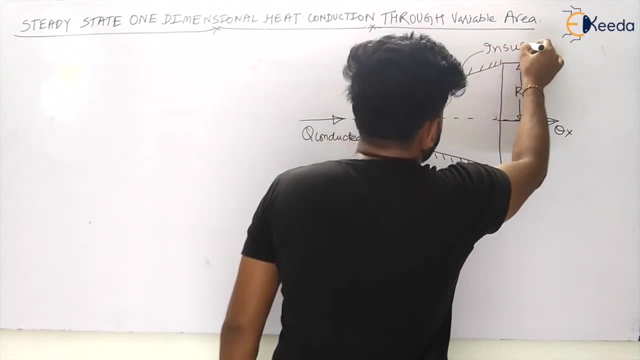 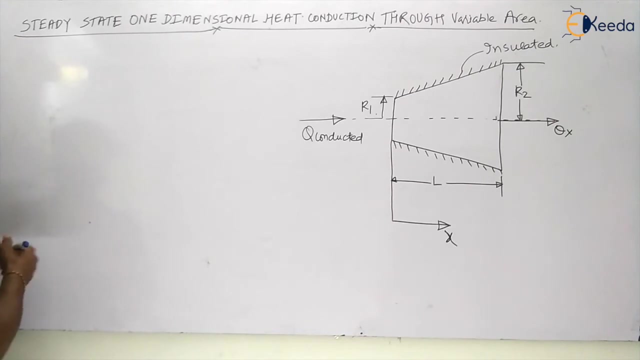 it. I will just insulate it, so the outer surface is insulated. this is your insulated radius students. So so there is one dimensional heat transfer. so can I see the assumptions here? yes, what are the assumptions? so, assumptions number one: already, given that is your steady state. 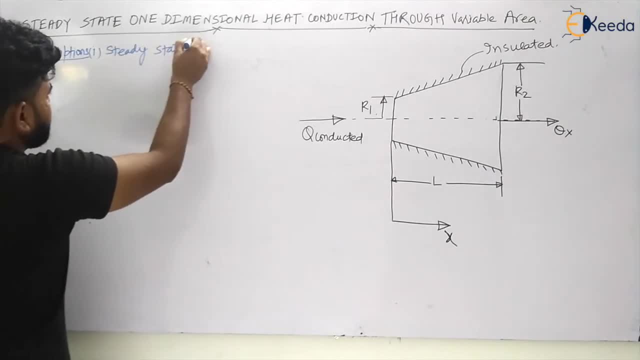 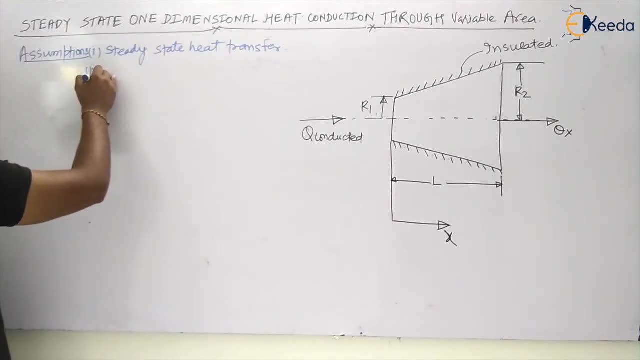 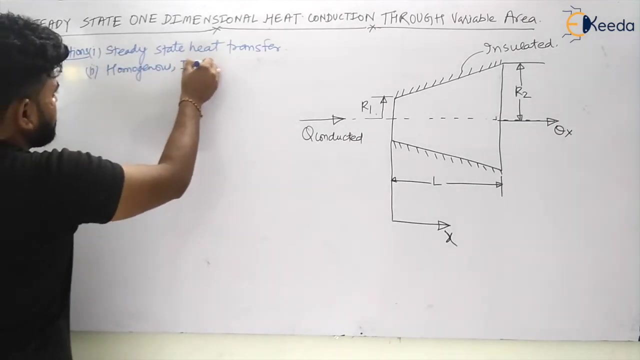 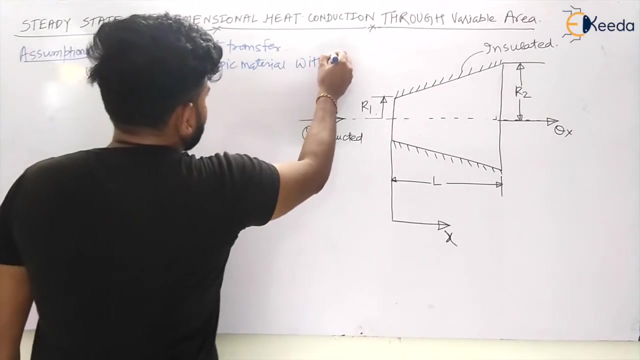 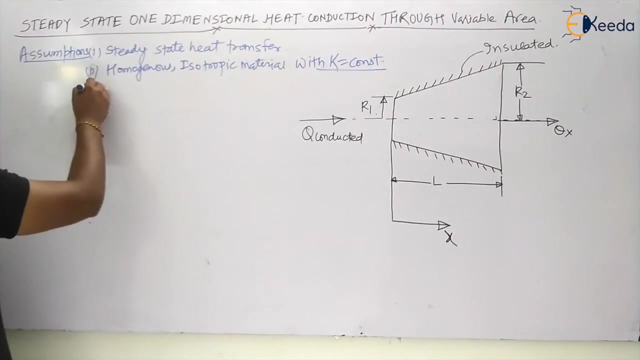 heat transfer: steady state heat transfer. what is your second assumption? second, is your homogeneous material. we have already seen homogeneous material, homogeneous isopropane, isotropic material with conductivity k is equal to constant. that is not independent. that is independent of the temperature. and the third one is: what I am assuming is there. 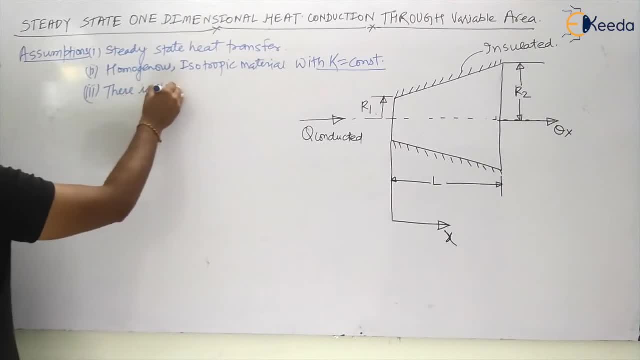 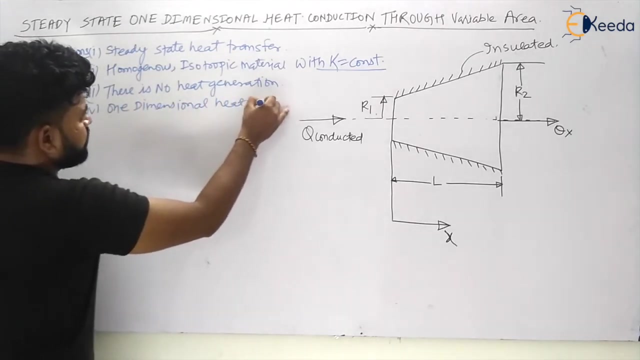 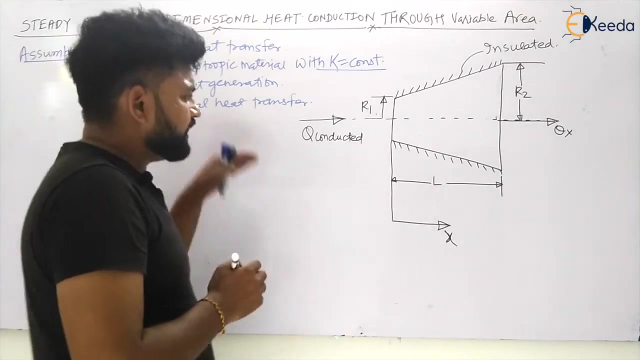 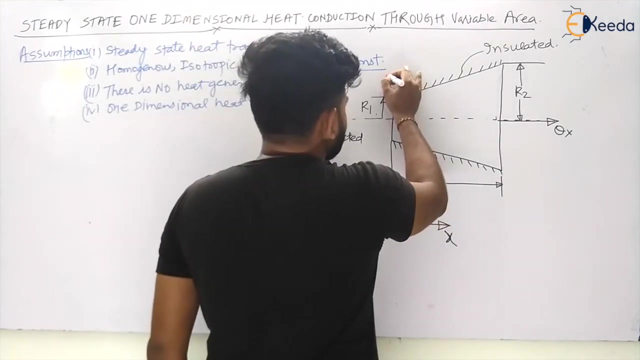 is no heat generation. there is no heat generation and one dimensional. we have already taken one dimensional heat transfer. So, my dear students, let us see, if there is a heat transfer in this particular variable area, slab like this, then there must be some high temperature here. let us assume that temperature. 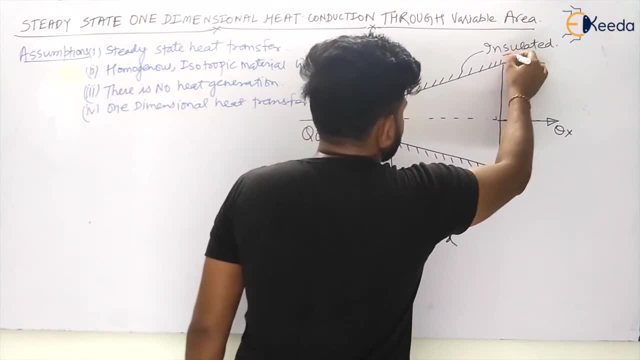 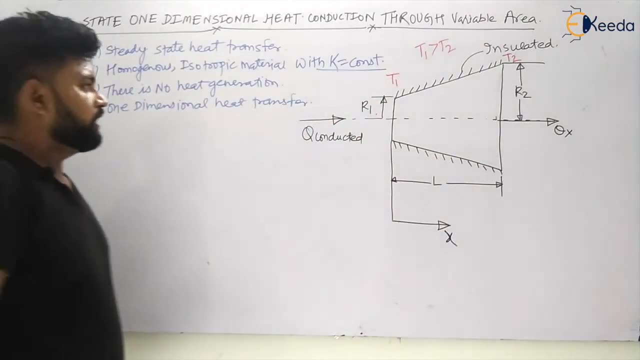 is T1 on this surface and temperature is T2 on this surface and T1 is greater than T2, okay, T1 is greater than T2, very good. Now let us consider a temperature. So let us assume that temperature is T1 on this surface and temperature is T2 on this. 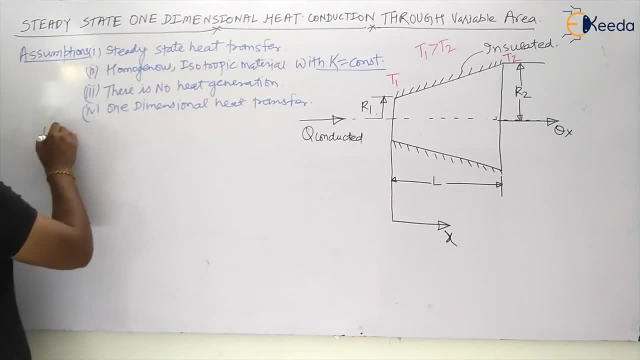 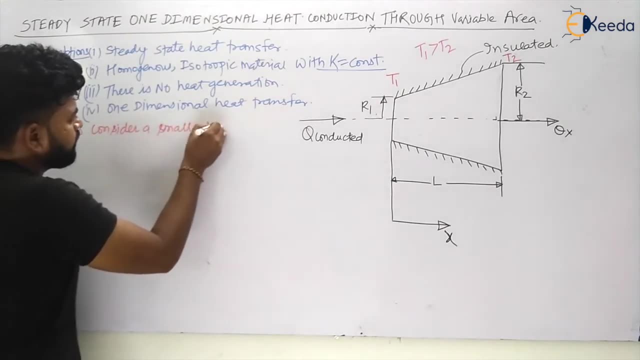 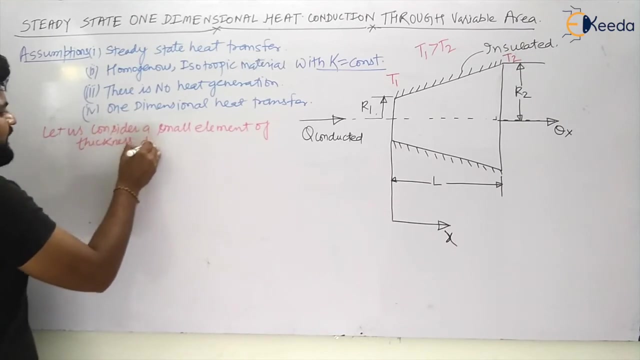 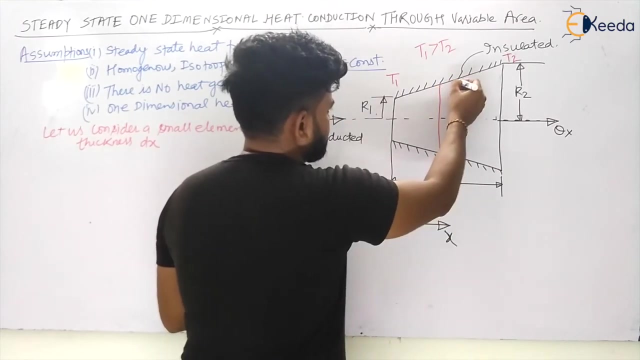 surface. okay, Let us consider a small element. So let us consider a small element of thickness of thickness, dx, dx. So what I am doing is I am considering an element. Let us see, this is your element. 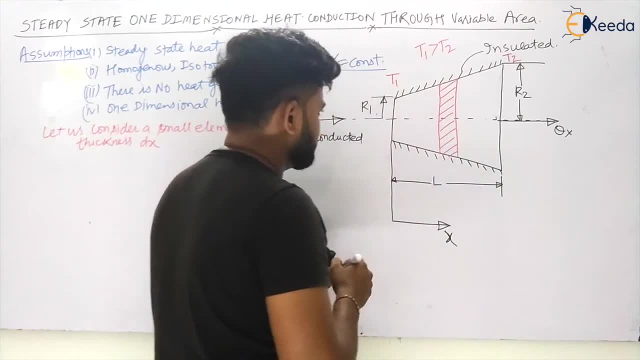 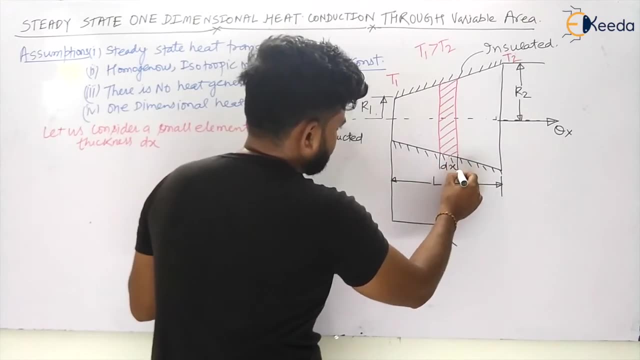 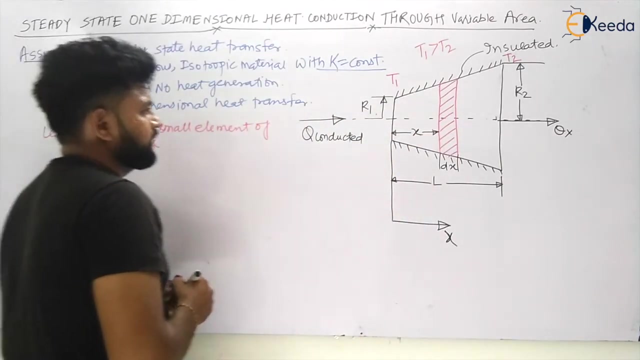 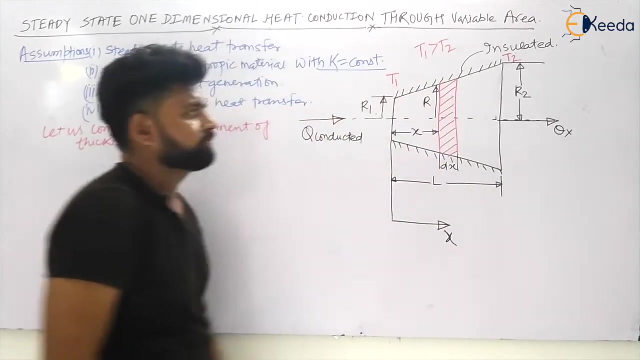 which is having x distance from that r1. so that is your dx and this is at x distance, apart from r1. okay, now, this is dx and let us say, this is your r. so what will be your r? can i calculate r here, my dear students? yes, i can calculate this r. 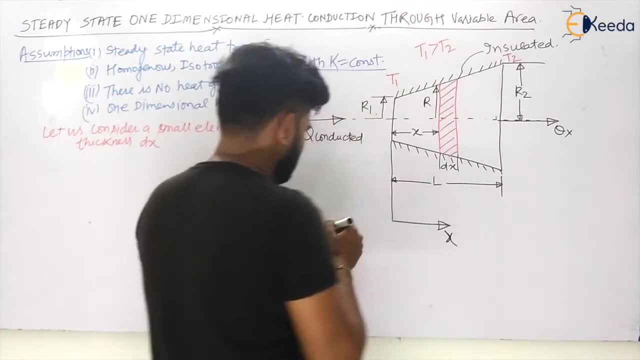 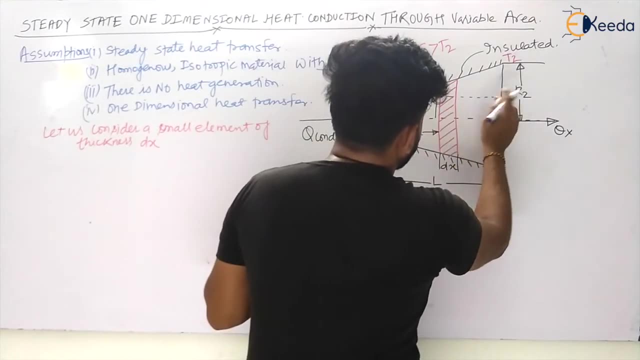 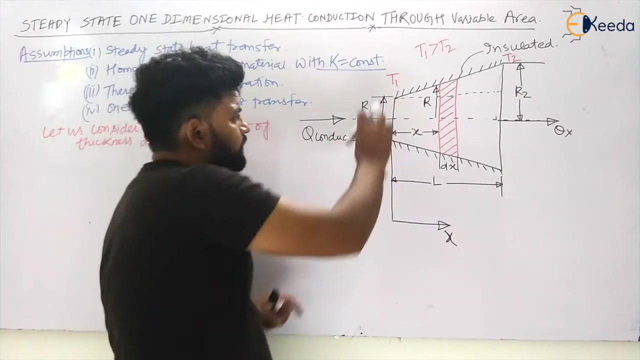 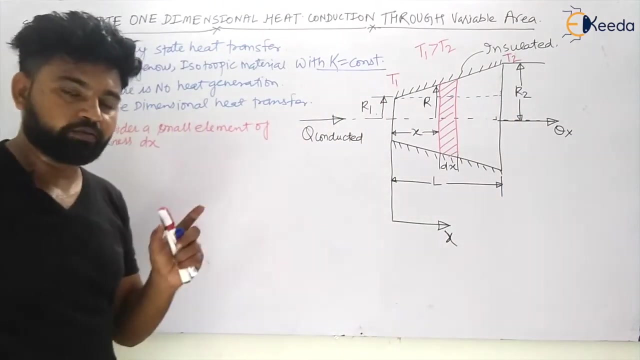 this r will be given by this r1. if i will see, let us do all the calculations, mathematical calculations. so if i will do like this, so, my dear students, there will be some- this will be r1 throughout. let us take. let us take that is r1 is constant throughout this. so there will be two concurrent. what triangles is there will? 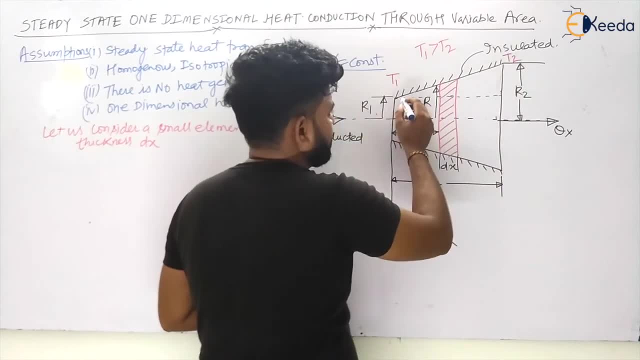 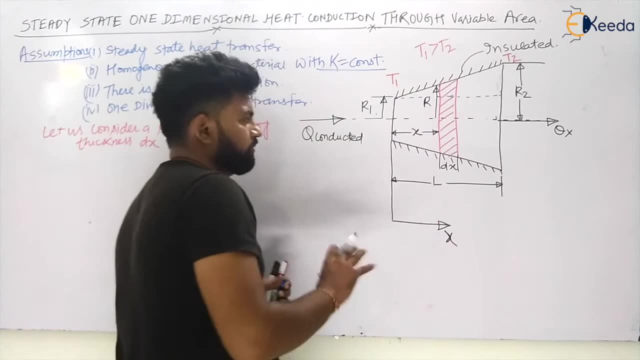 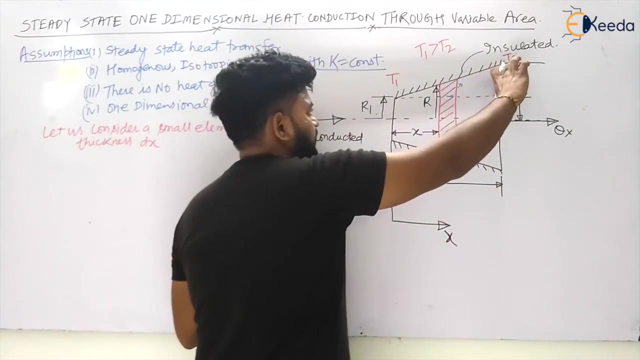 this triangle first, and there will be what again? there will be this triangle and there will be this triangle, this triangle, this one. so can i have dynalogy between them? yes, so this r and this is what this is, how much this will be, how much this will be r2 minus r1. so this distance will be nothing but your r2 minus r1. 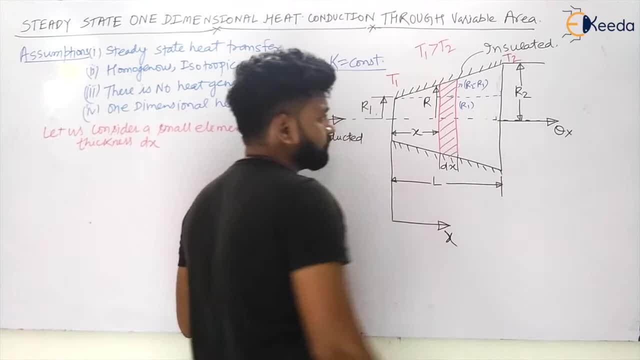 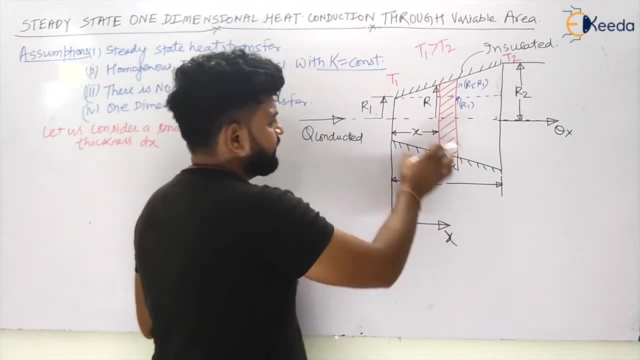 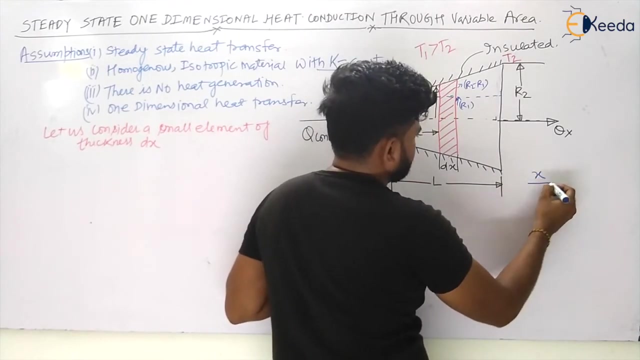 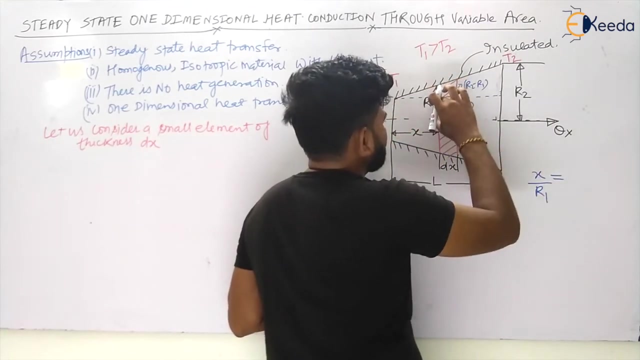 and this will be your r1 and this will be your r1 up to here. up to here, okay. so this will be length l and this will be x. this will be length l, this will be x. so what i can do is i can take that x upon r1 is equal to x upon r1, x upon r1, so it is not r1, it is r2 minus r1. 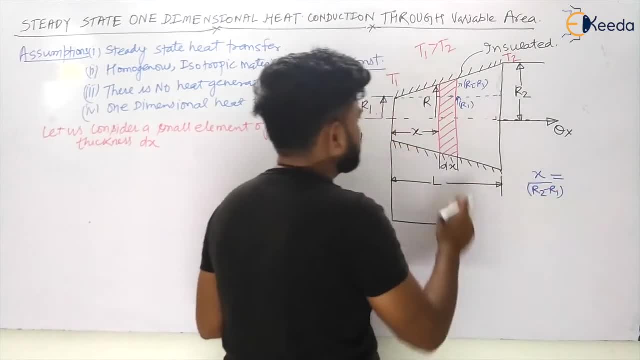 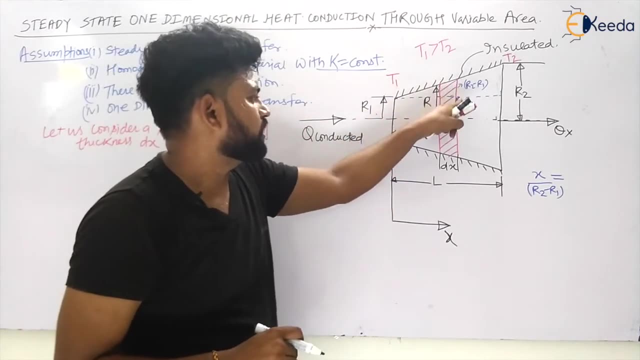 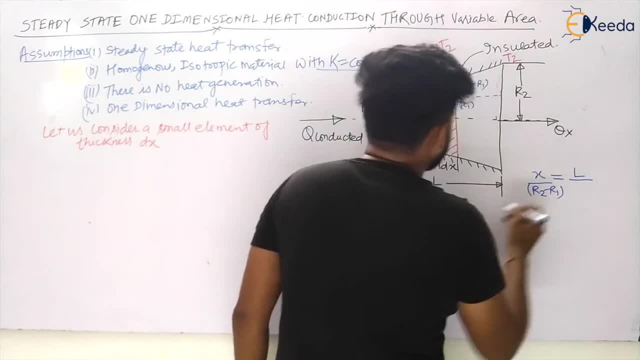 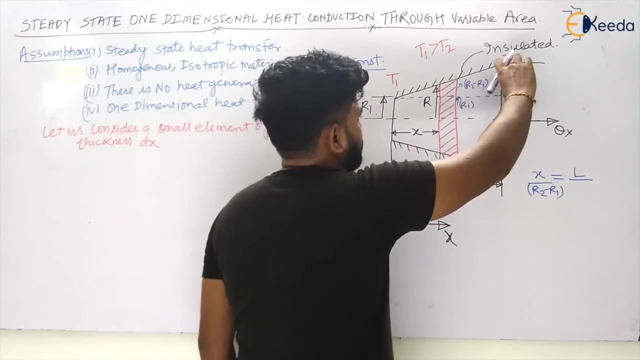 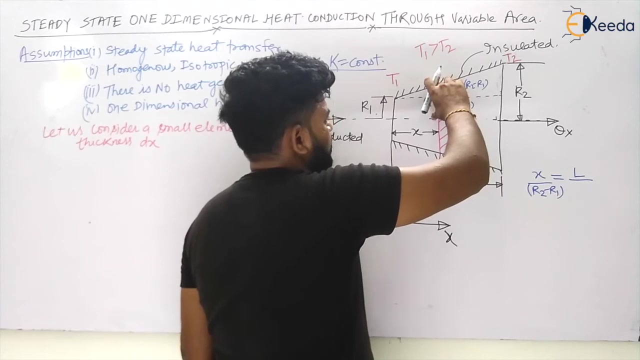 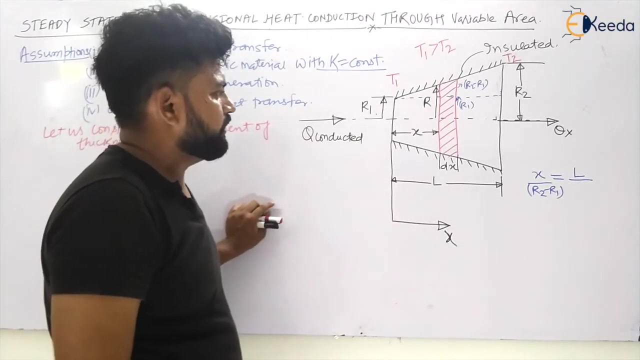 and this will be equal to l upon. this will be equal to l upon. that is your l for the bigger triangle, l upon. this will become how much this will be r2 minus r1, and this will be what- r only, r only. so let us see how it will be. so this will be r2 minus r1 divided by r1, so this will be given. 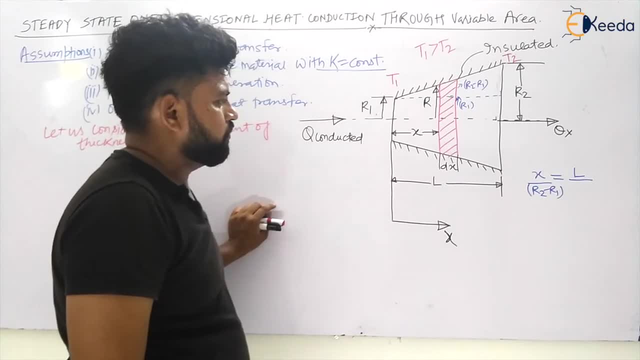 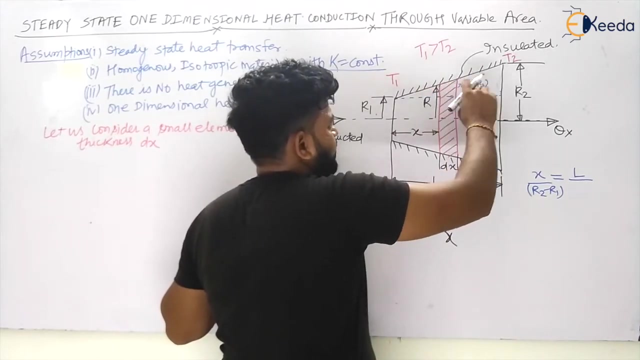 by this will be your r, and we have to calculate only this distance, first of all this distance, because we know r1. so this triangle and this triangle, so this will be r2 minus r1 x upon r2 minus r1. so this will be r2 minus r1 x upon r2 minus r1, so this will be r2 minus r1 x upon r2. 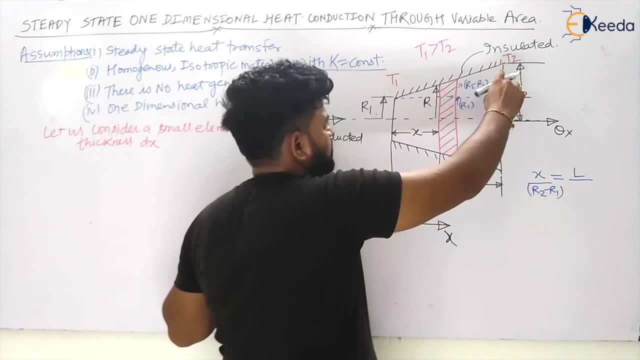 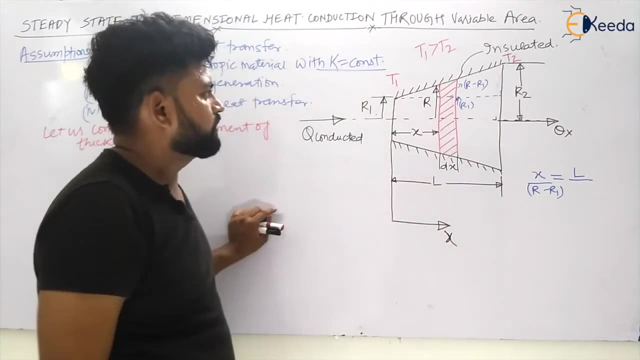 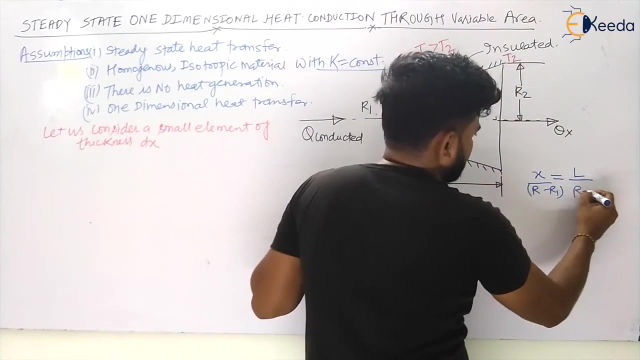 and for this bigger triangle, this will be r2 minus. so this is r minus r1. r minus r1, this will be r minus r1, my dear students. okay, r minus r1. so that is capital r. that is r1. that is capital. r2 minus r1. so l upon r2 minus r1, my dear students. so x will be equal to nothing, but. 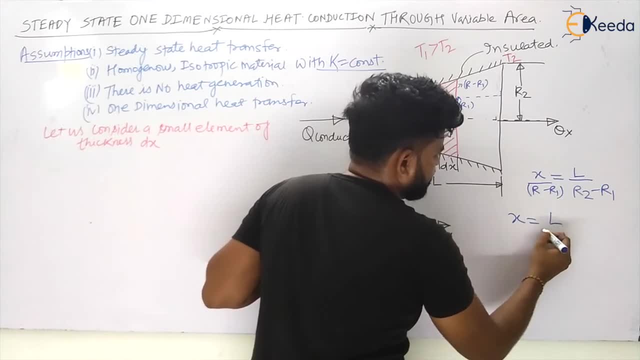 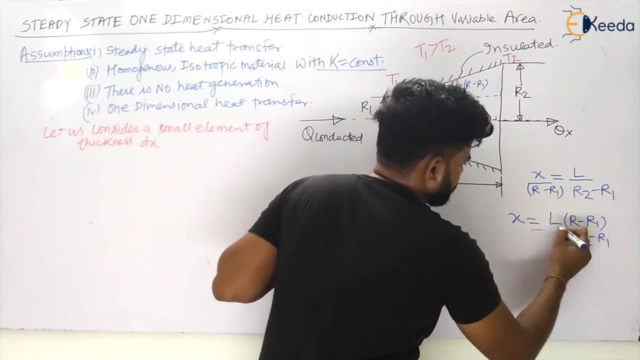 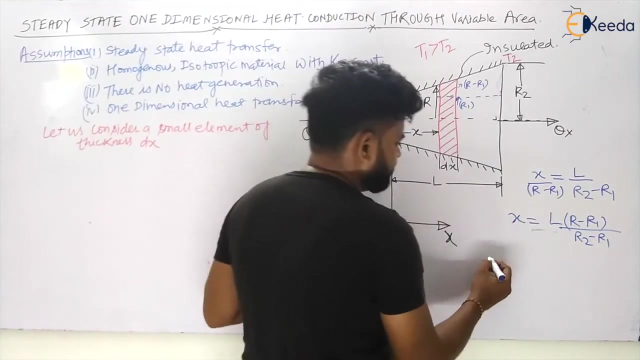 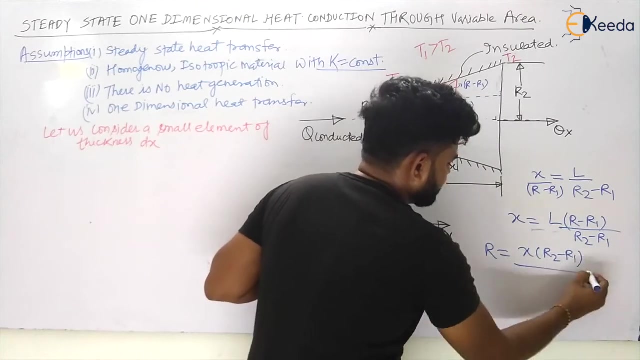 your l upon l into r minus r1 upon r2 minus r1. okay, this will be your x. so can i have r from this equation? can i have r from this equation? so r will become equal to x into r2 minus r1, divided by, divided by l, divided by l plus. 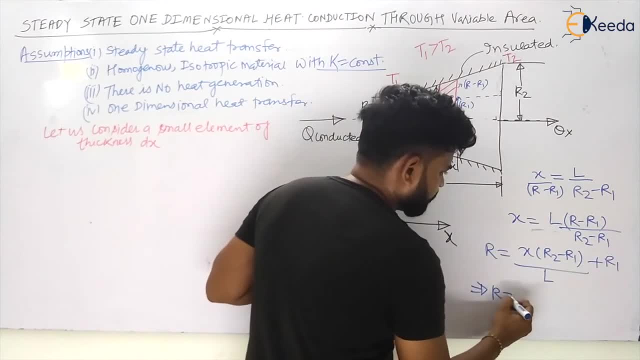 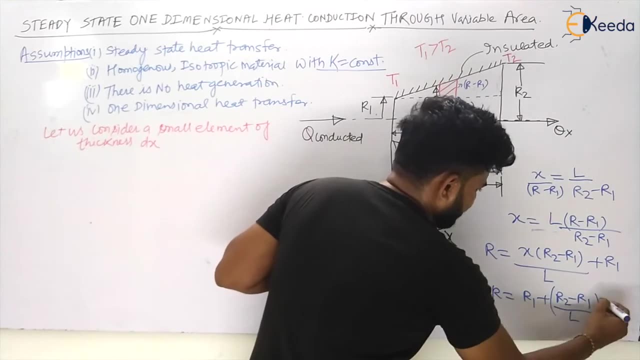 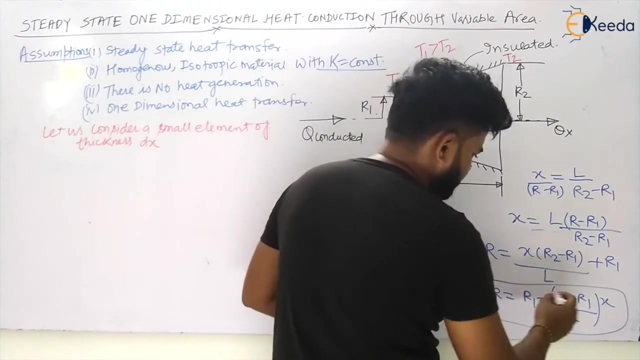 r1. so this will become: r is equal to r1 plus r2 minus r1, divided by l, into x, into x. so let us take this value to be c constant c. let us take this value, r2 minus r1 by l, to be some constant for. 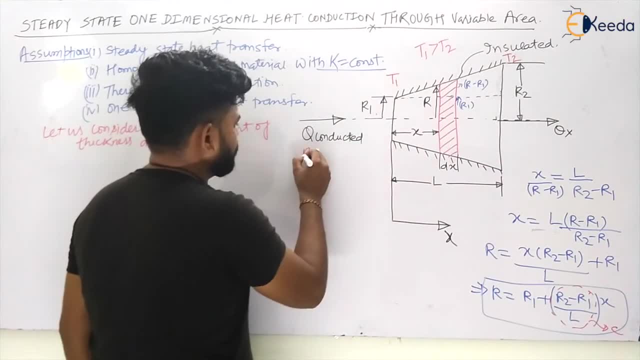 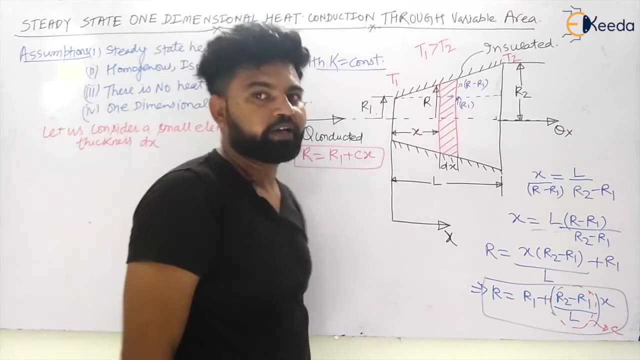 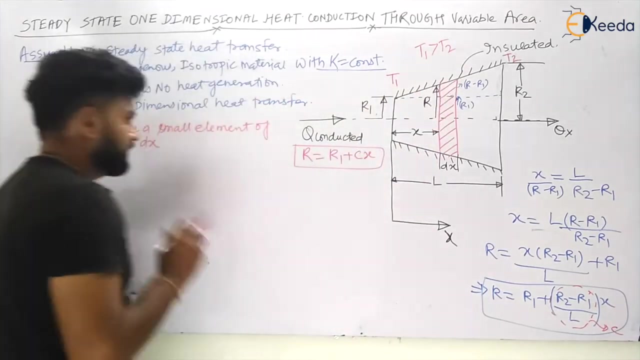 easy calculation. let us see so your r will become equal to how much r1 plus c x. so now we know r for that particular element, we know r for that particular element. my dear students, i think you have understood the concept of congruent triangles, that is, the concept of ninth class congruency. 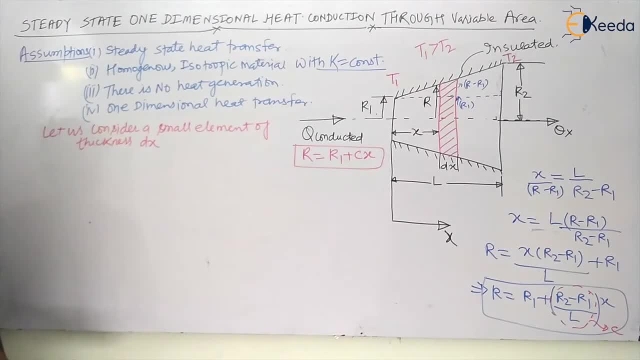 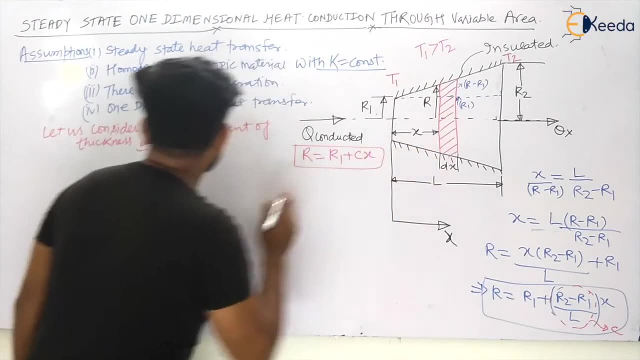 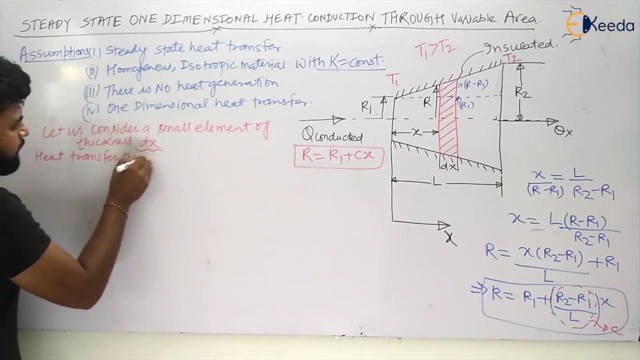 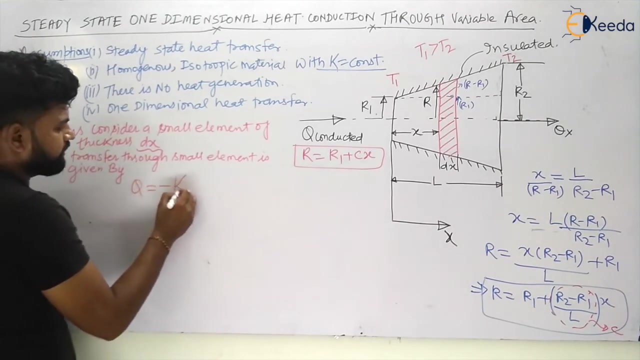 of triangles. let us consider a small element of thickness dx. okay, thickness dx, so can i have the heat transfer through this area, through this small element? so heat transfer through small element is given by, heat transfer through through this small element is given by given by what this will be given by. q is equal to minus kappa k, that is conductivity of. 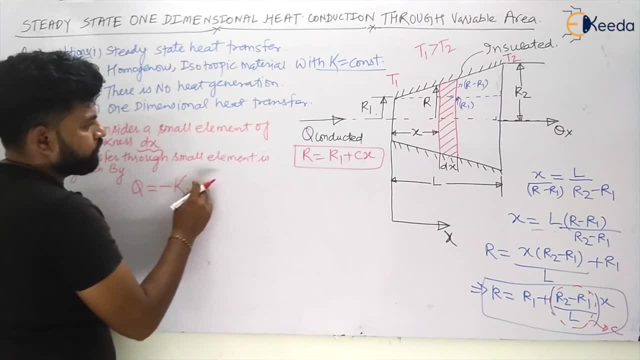 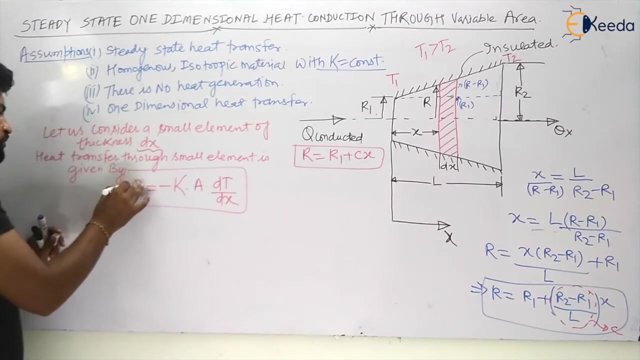 that element into area. so what will be the area? area will be varying, so area will be varying. so X, k, that is conductivity of that element into area. so let us take it dq. So if I know the heat transfer, because it is characteristic heat transfer, so the heat transfer will be Q only. 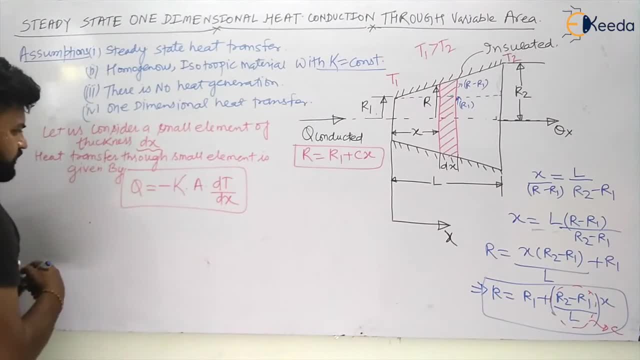 I don't have to worry about anything. Let us see. Let us do it with my dear friends. So if I will take dx this side and area this side and k will take this side, only Let us assume the conductivity is k for this, because I have not taken. 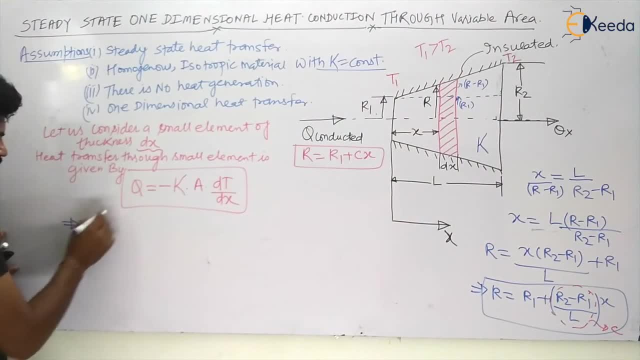 Now, what will be the heat transfer? Let us see So Q into dx. this side I am taking. this, Divided by area A, is equal to for that small element I am talking about minus kappa A- into dt. So if I will integrate it both side, 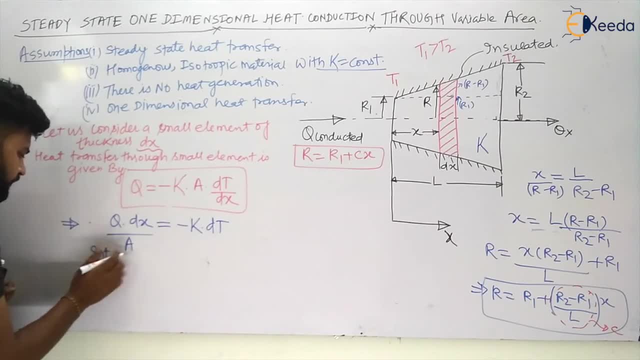 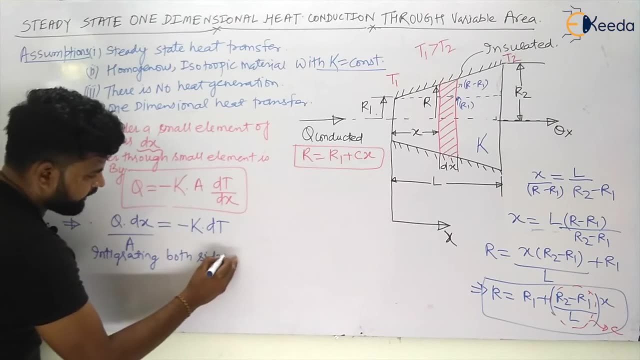 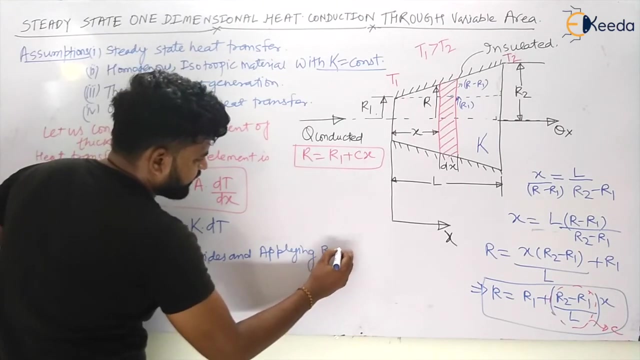 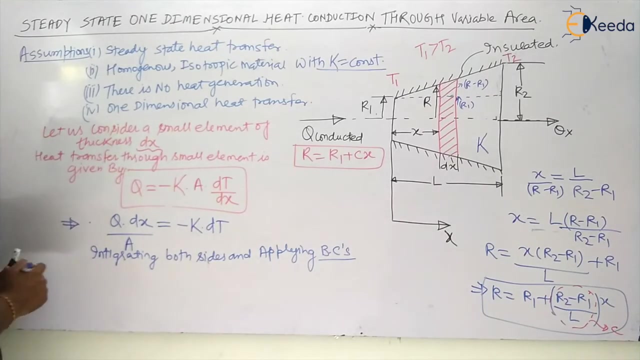 So, integrating both side, Integrating both sides And applying boundary conditions And applying Boundary conditions. So we will see boundary conditions, Don't worry. So, applying boundary conditions, What we will have, We will have that Q into dx, divided by area, which will be nothing but what? 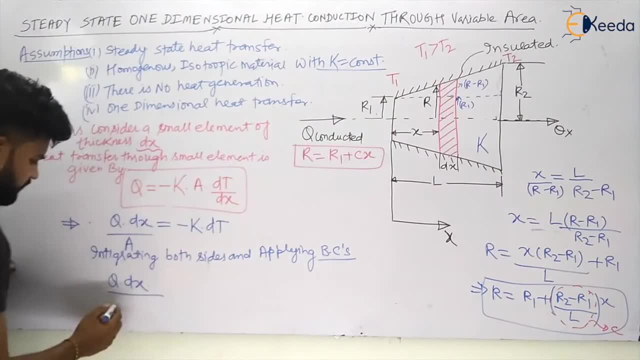 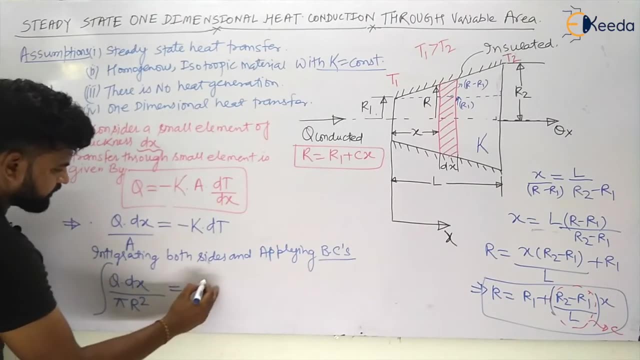 What will be the area for this circular element? This will be nothing but your pi r square, Pi r square. So integrating this is equal to minus k into dt, And again integrating this. So I will have something. Why? Because I am integrating this. 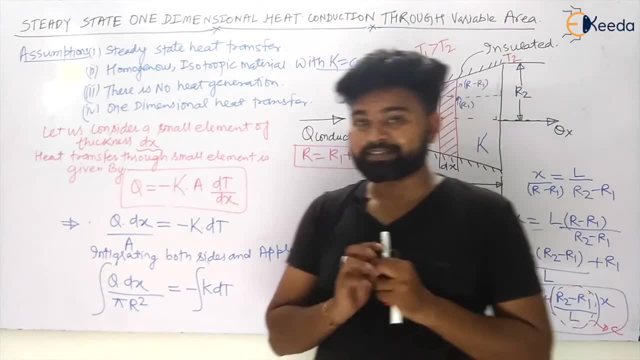 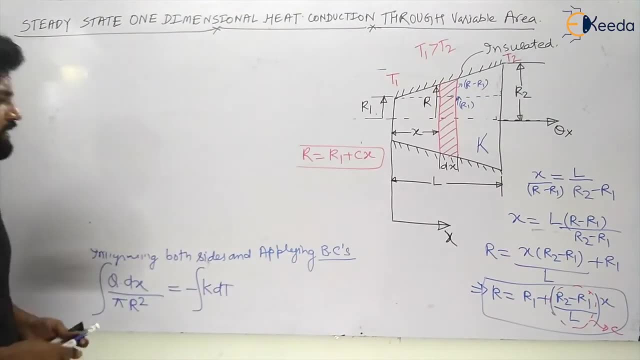 So I can easily calculate the heat transfer. then, For the variable area, Let us see, Let us see. Let us see it Now. so, my dear students, I know that r is equal to r1 plus cx. Can I put the value of r here? 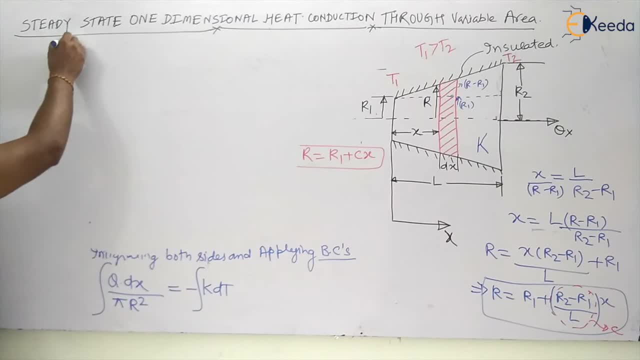 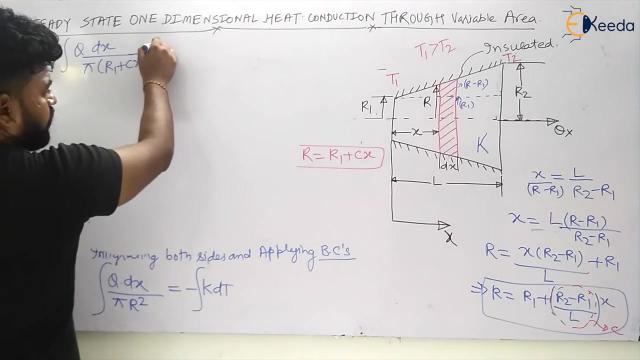 Yes, So putting the value of r. So what I will have? Integration of Q into dx, divided by pi into r, which is nothing but what? r1 plus cx square, cx, r1 plus cx square Is equal to minus k. integration of dd. 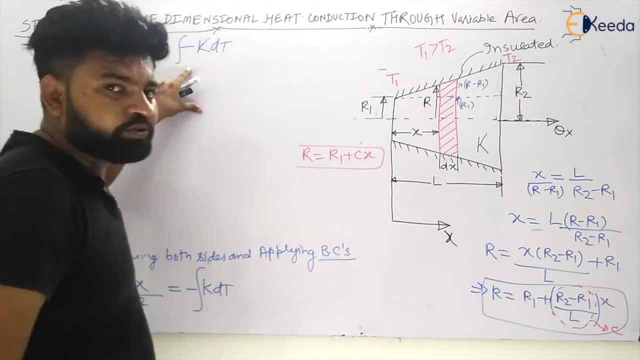 dd. So what are the boundary conditions? Let us see. First of all, I should integrate- Okay, Let us integrate it, But first of all I should know the. what are the boundary conditions? So r will be from r1 to r2.. 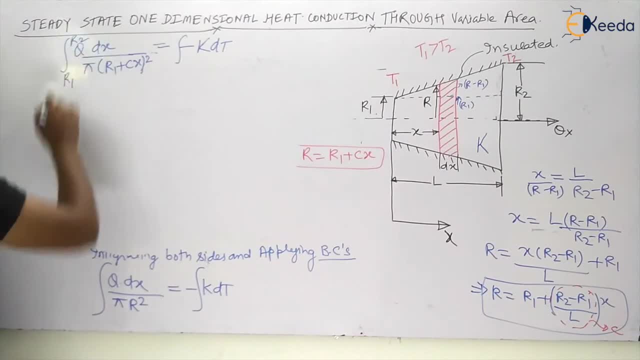 So this will be from r1 to r2.. Or I should take x, I think, Because I am integrating this. So this will be 0 to l, not r1 to r2.. This will be 0 to l. 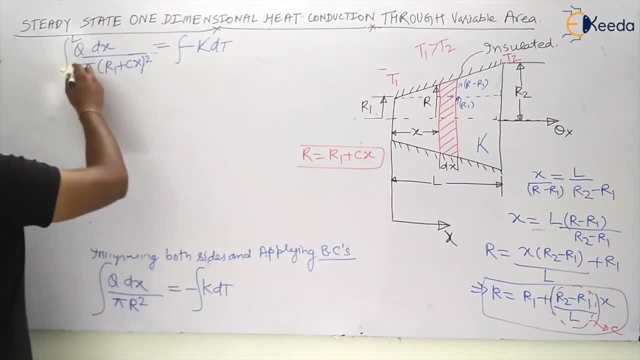 0 to L. okay now, and this must be t1 to t1 to t2, t1 to t2. let us indicate, guys. so what will be there? let us see. so q, dot, dx, so q I can take out and pi I can take out, because these both are constant, so I can have the integration of dx upon r1. 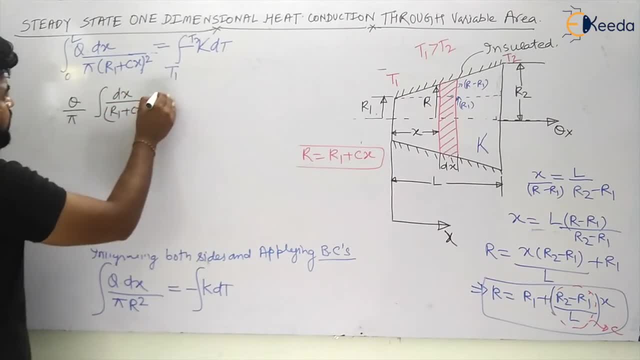 plus cx square. okay, is equal to t1, to t2 minus k dt. so now, integrating what I will have, let us see q by pi. integrating this, what is the integration of dx upon x square, dx upon x square? so this will be nothing, but what this power will be. 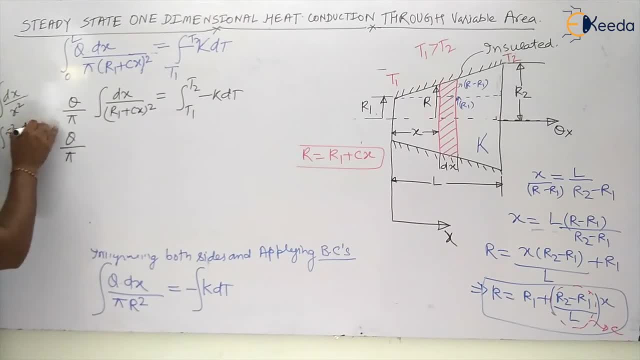 nothing but x. square to the power minus 2 into dx, so this will become x to the power minus 2 plus 1 divided by minus 2 plus 1. so this will be your integration. though this will become x to the power minus 1 divided by minus 1. this will become minus 1 upon x. so 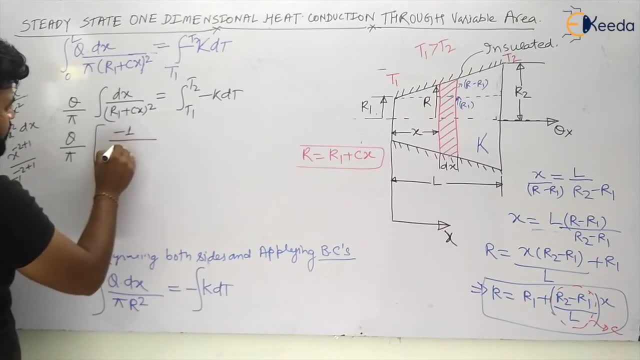 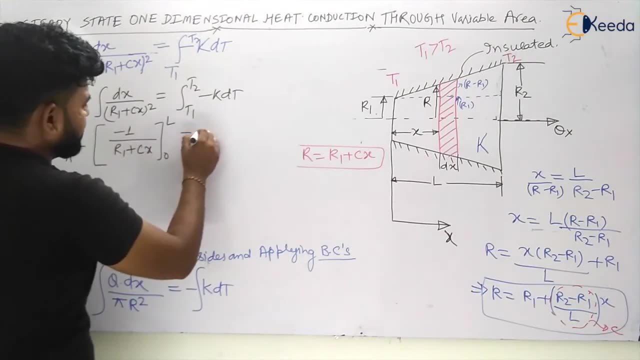 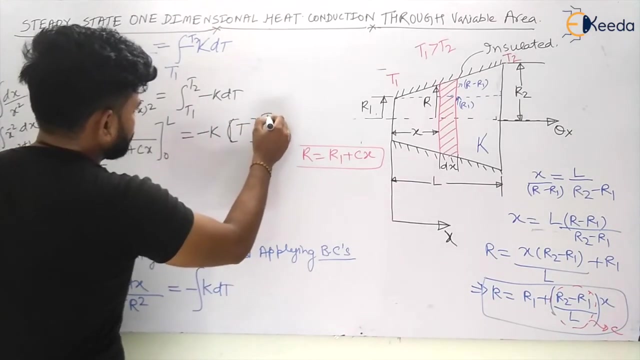 minus 1 upon x will be your integration. so minus 1 upon r1 plus cx will be your integration, and this will be 0 to L. so here I will have minus k kappa into temperature. this will become t to the power, t1 to t2. so let us put all values. 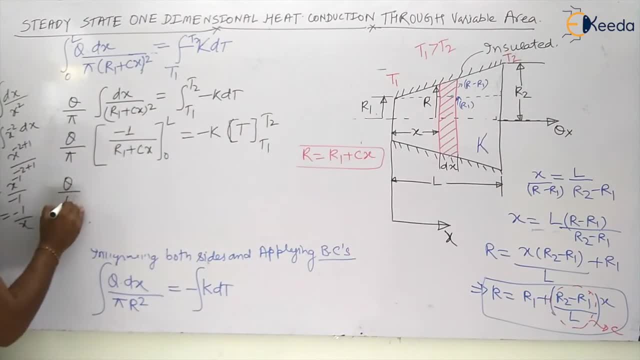 if I put L here, let us see what will happen. so q by pi. so okay, there will be some one integration of cx. c part will be there. so if you will do the integration of that c, this will come down side by their strengths. this will come 1 upon c. also, when you will do the integration of what cx, then what will be? 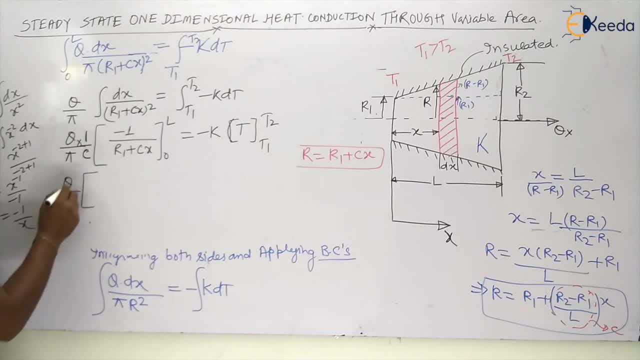 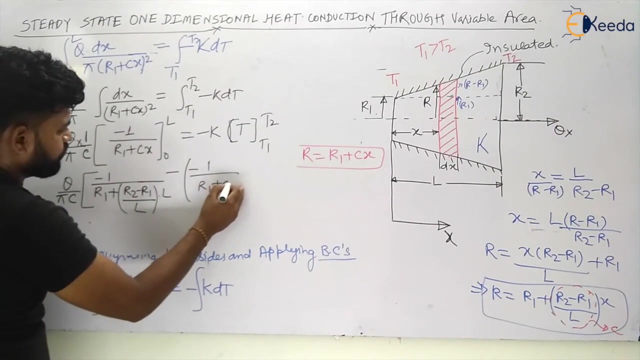 this, this will become 1 upon c. okay, now this will be pi, because c is a constant here. so q upon pi c. this will become minus 1 upon r1 plus c. what is c? r2 minus r1 upon l? and we are putting the value of x here. let us see l minus of minus 1 upon r1 plus c into 0. 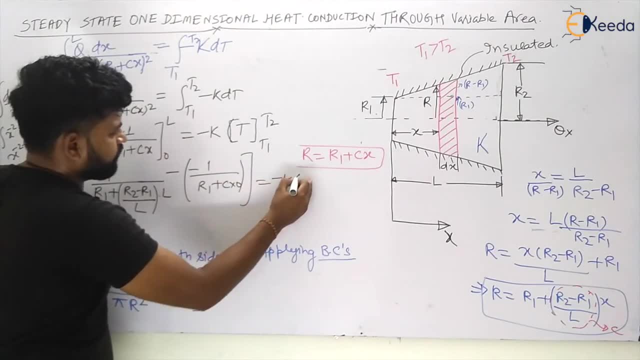 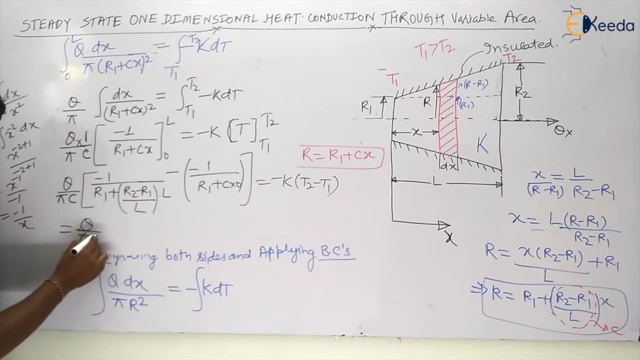 c into 0 is equal to minus k of e to minus e1. okay, my dear students, let us see. let us see here. so now, q upon pi, c will become equal to, so r1. l l will go, so r1, r1 will go, so this will become. 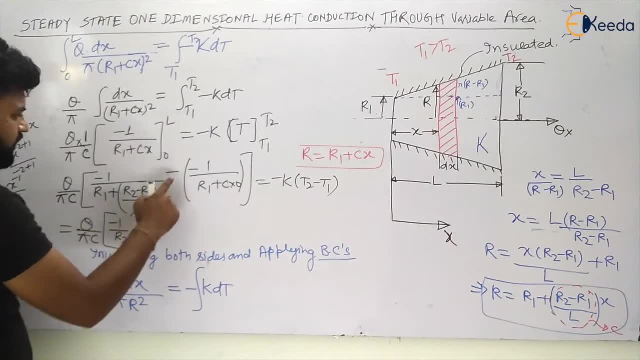 1 minus 1 upon r2, minus 1 upon r2, minus minus plus, this will become what, 1 upon r1, 1 upon r1, is equal to minus k of t2 minus t1, minus k of t2 minus t1. so let us see. let us see. 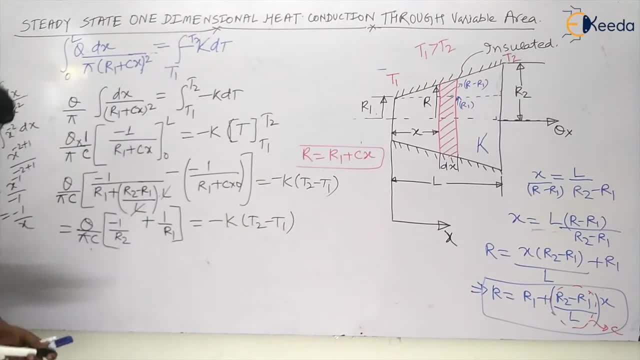 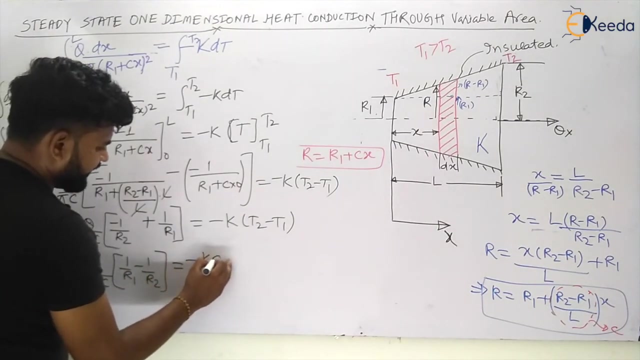 so this will become your. this will become your what? so this will become your: q by pi into c, into 1 upon r1 minus 1 upon r2. okay, my dear students, and this will become this side. k a, delta t. we can directly take k a. 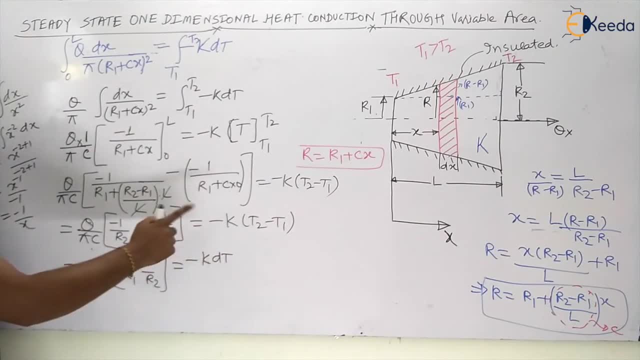 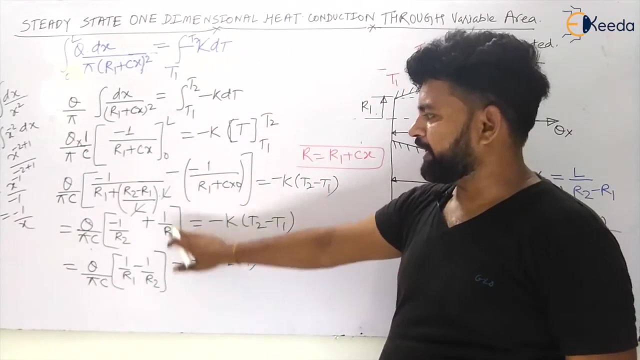 delta t minus of k dt, that is, t2 minus t1. so delta t we will like later, because let us take it right like this only. so, my dear students, i think you are getting the concept. i think you are getting the concept. so we have put all the values of l and 0, that is, that was. 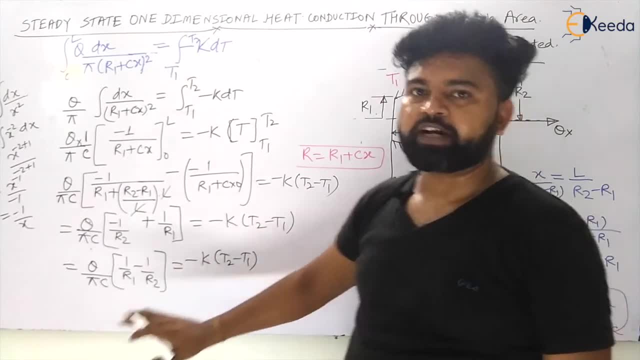 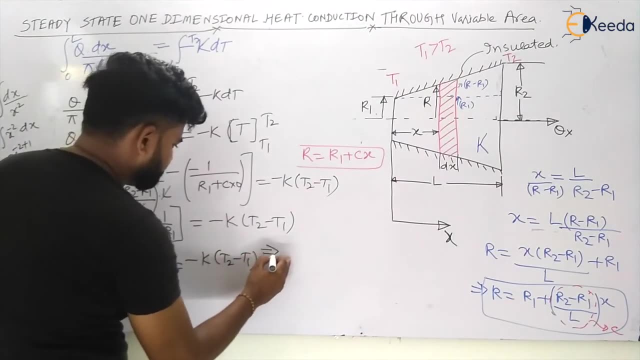 varying from 0 to l, and we are getting this equation. now let us find it. find out what will be the heat transfer. so if i will take this, so this will become how much, let us see. so this will become q upon i am putting the value of c. i am putting the value of c, that is r2 minus. 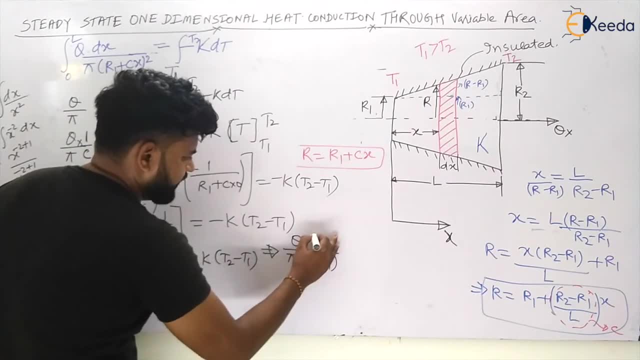 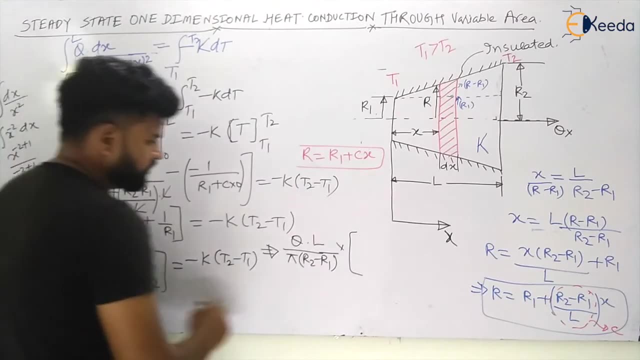 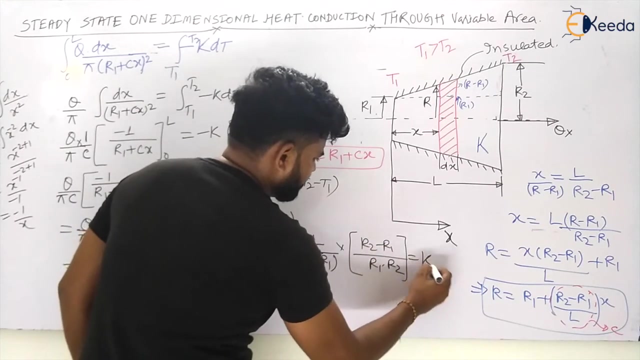 r1, r2 minus r1 divided by l, r2 minus r1 divided by l. now multiplied by, if i will take that deltium of both these, so this will become r1, r2 and alpha side this will be r2 minus r1 and this will be equal to k minus of k into t2 minus. 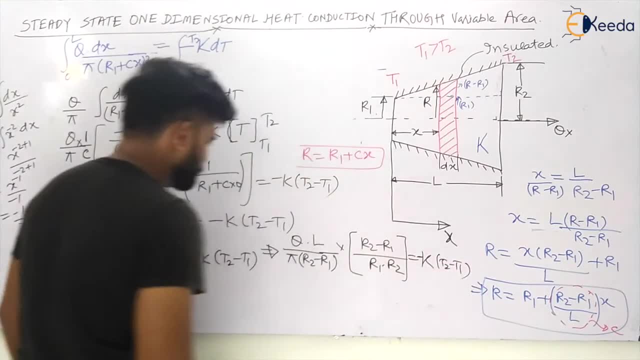 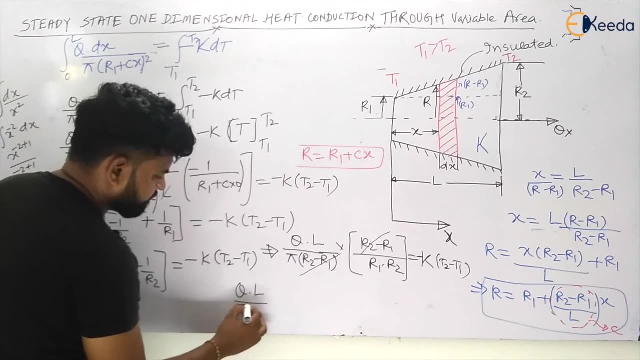 t1. okay, my dear students. so r2 minus r1 will go. so the remaining part will be q into l upon pi, q into l upon x, divided by r1, r2, r1, r2, divided by r1, r2. okay, okay, what will become? 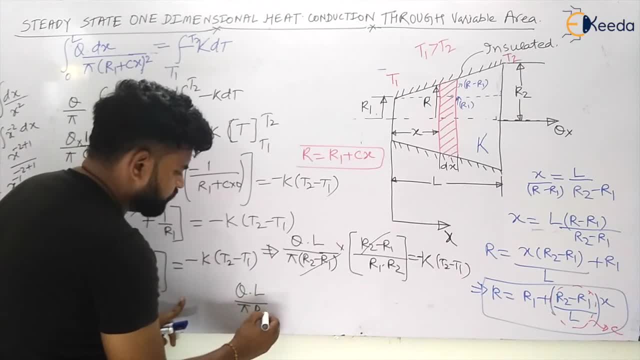 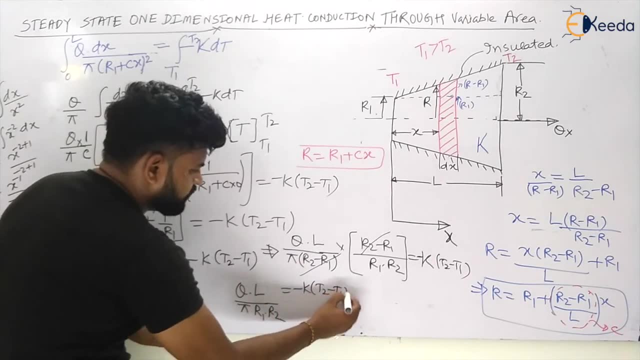 be q into l quantity. so if you modify that you will be able to find theMich Clnegite regression is equal to minus k, t2 minus t1.. So let us take this t1 inside, So this will become t1. 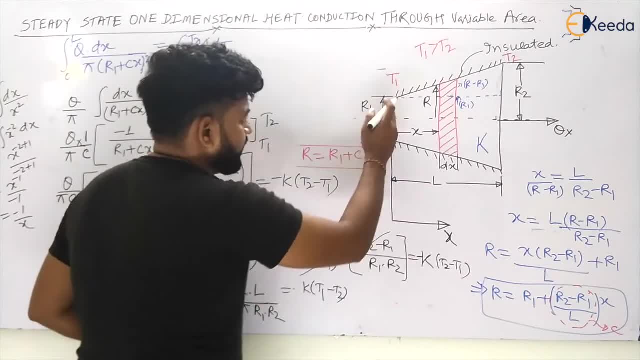 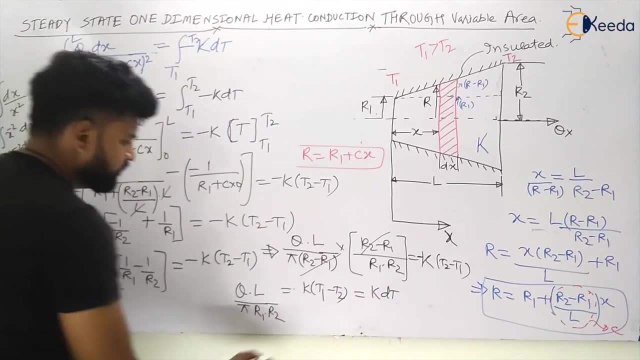 minus t2.. t1 minus t2.. So from higher to lower. So I can write dt now, So it will become k dt now. So what will be the heat transfer, my dear students? So q will be given by 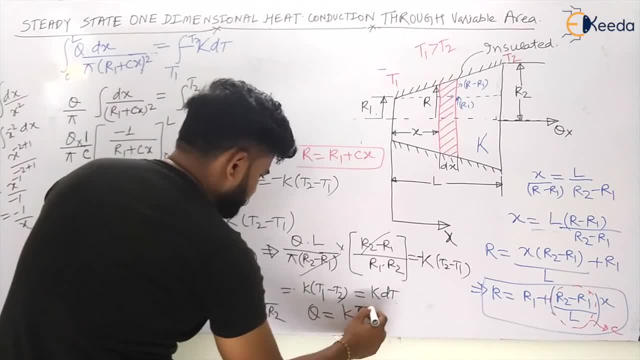 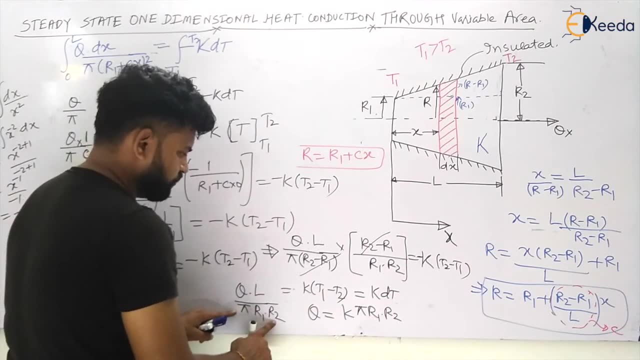 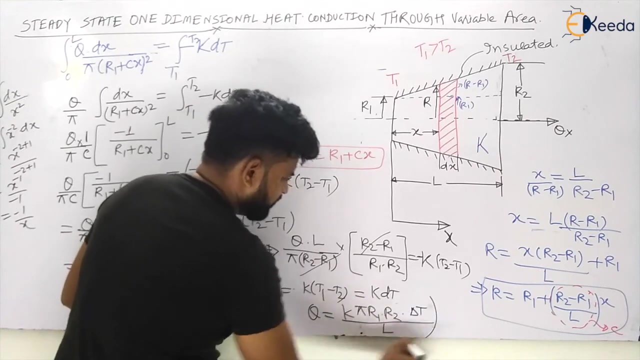 equal to k into pi into r1, r2, k pi into r1, r2 into delta t divided by L, Divided by L. So this will be your heat transfer and this is given by how much. Let us say I am writing here. 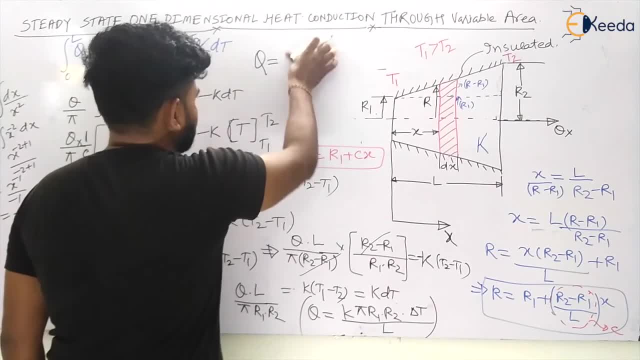 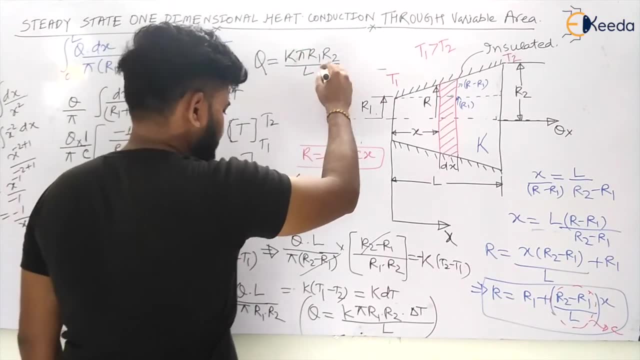 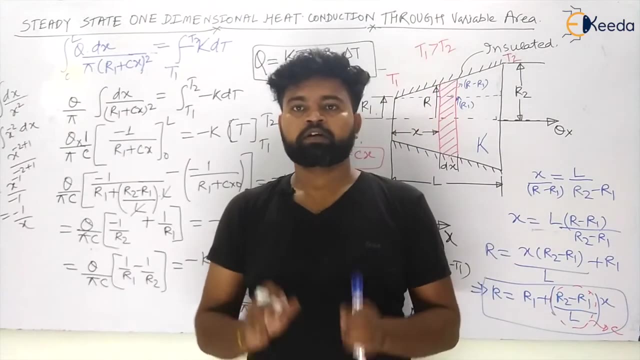 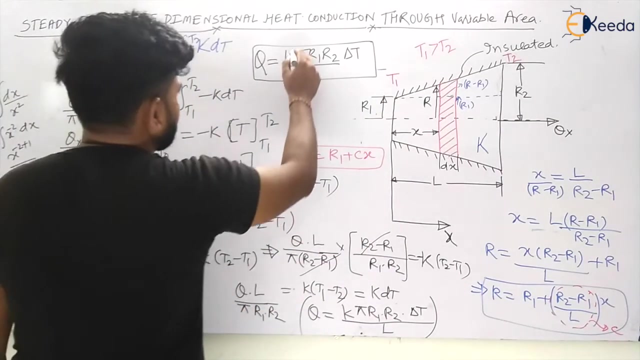 q is equal to pi, that is, conductivity k, pi r1, r2 by L into delta t. So this will be your variable. this will be the heat transfer for variable area. variable area: this will be the heat transfer for variable area and this is simple, You can easily take it. 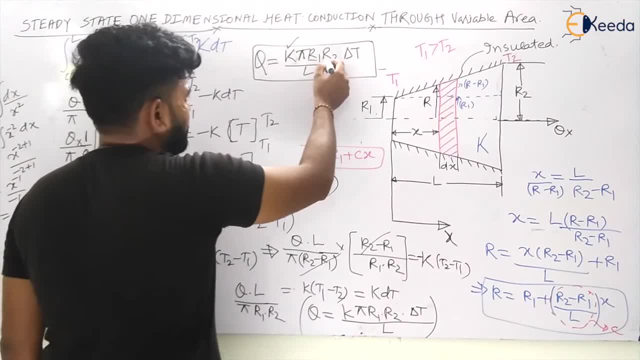 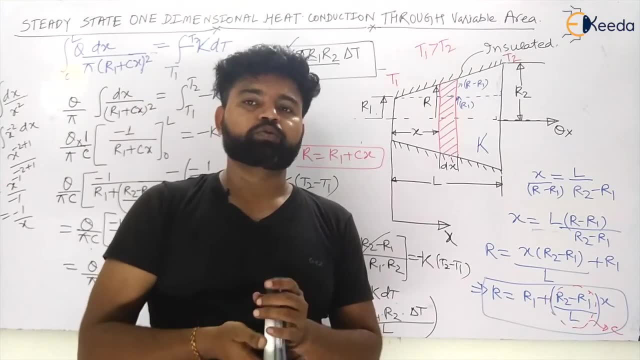 That is, pi into r2 must be there. So here it is r1, r2 divided by L delta t. So this was the derivation for your heat transfer or conduction through a variable area. Okay Now. so, my dear students, 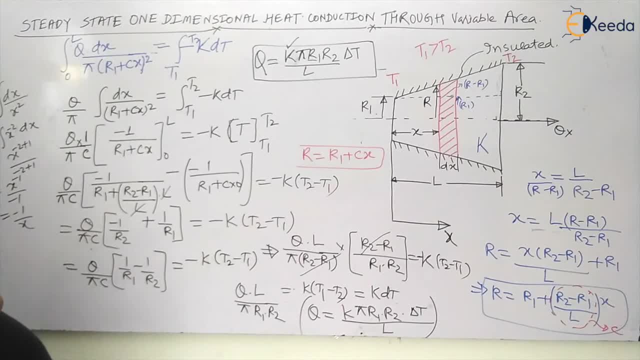 I think I hope you have understood the all set. So let us say temperature at any section x from the inlet. So can we have the temperature at any section from inlet, Can we have a temperature from any section at inlet. So let us calculate it. 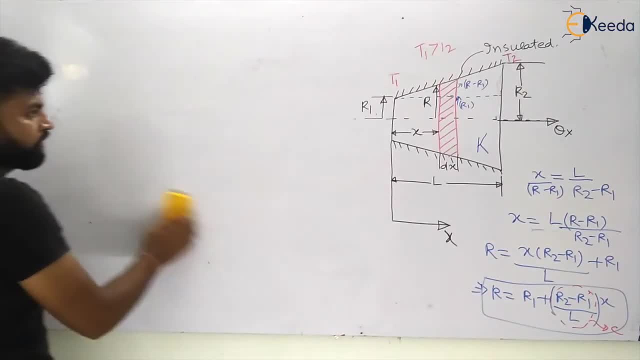 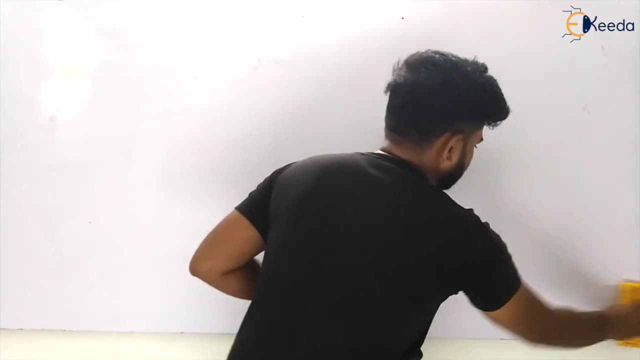 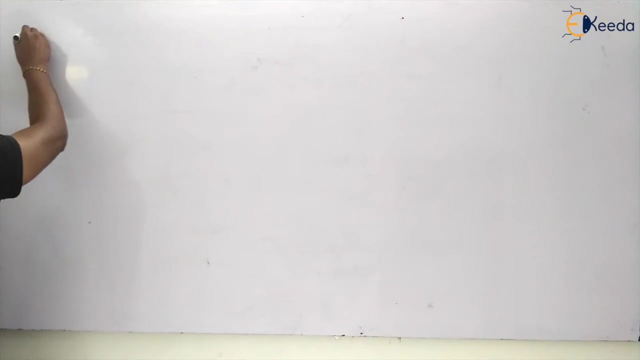 Or we can say: inlet is given by how much? Let us see. So, my dear students, I have to calculate now, the temperature at any section through variable area. I have to calculate temperature at any section from the inlet. So temperature in variable area. 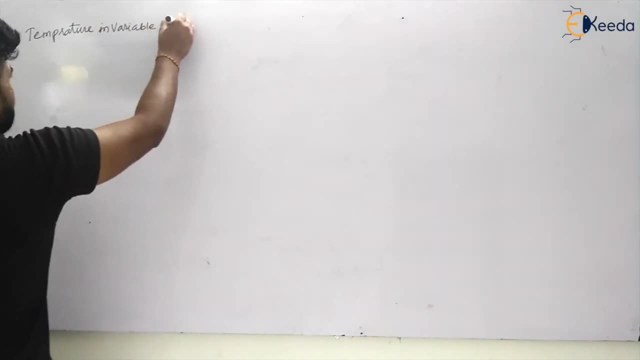 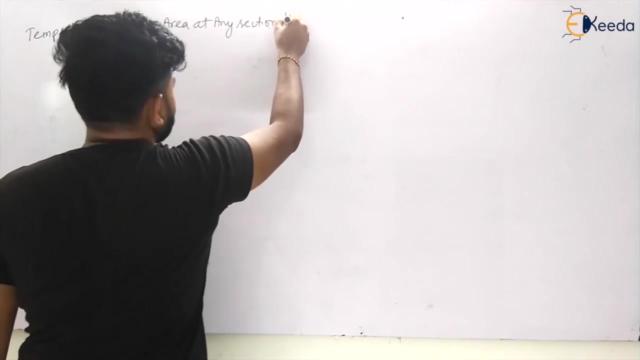 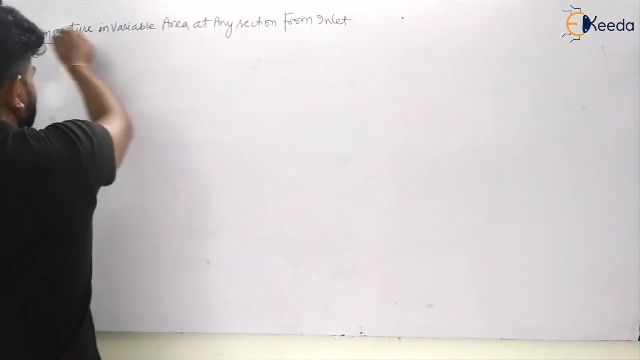 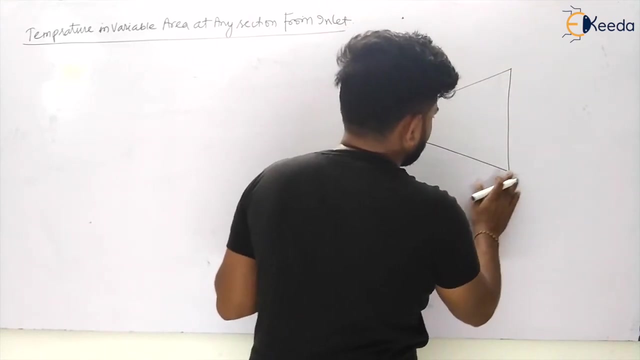 at any section from inlet, From inlet: Okay. So let us see What will be the temperature through this inlet. So this is your variable area, my dear students. So this is your variable area, my dear students. So this is your variable area, my dear students. 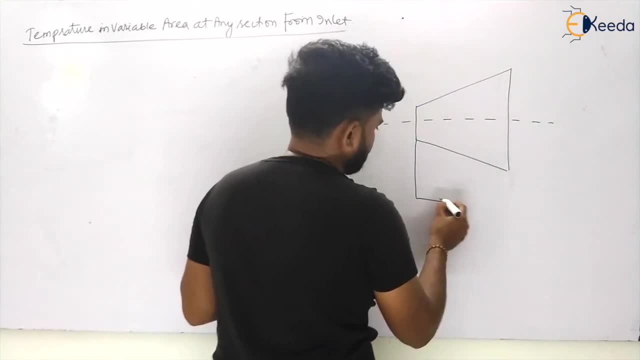 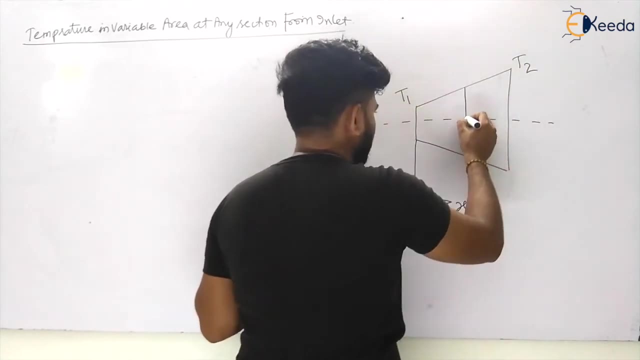 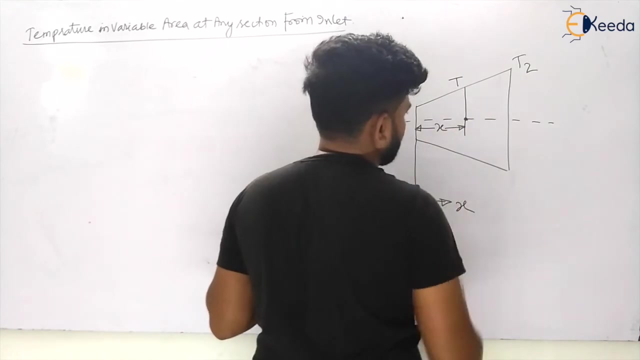 So this is your x in this direction. And let us say: temperature is t1 here, temperature is t2 here. So I want to calculate temperature t here at the distance of x, At the distance of x. Let us take the length of this. 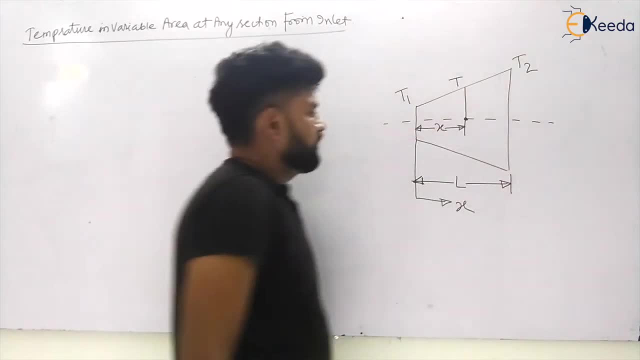 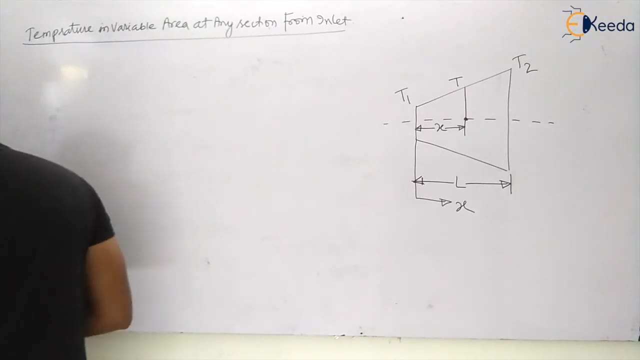 particular variable area, L. Length is L, So can I calculate the temperature at any cross section. Yes, I can calculate the temperature. Let us see how. So at x equal to 0, what is the temperature? So at x equal to 0, what is the temperature Can I calculate? 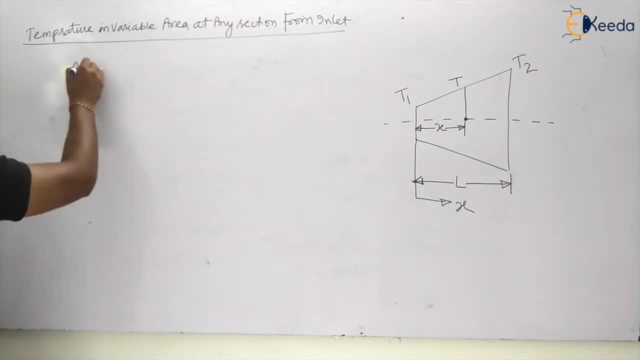 So, at x equal to 0,, the temperature t is equal to t1.. At x, temperature t is equal to t. At x equal to L, temperature t is equal to t2.. So these are the boundary conditions you know. 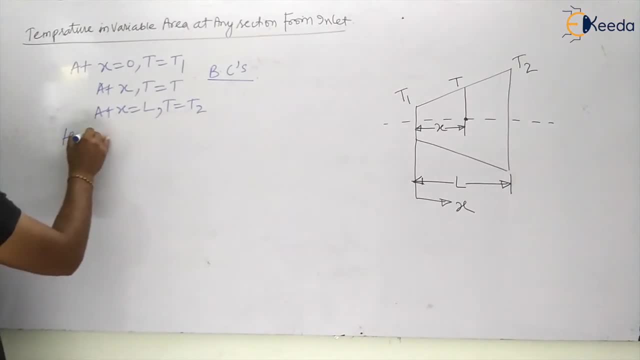 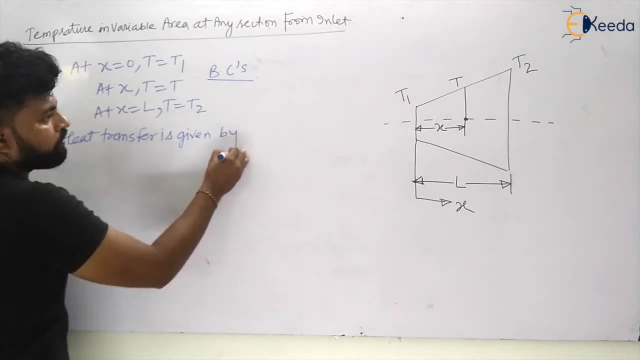 You already know. So what is the heat transfer given by? So heat transfer is given by, is given by how much. So heat transfer through this variable area is given by Q, And that Q will be equal to nothing, but equal to kappa A. 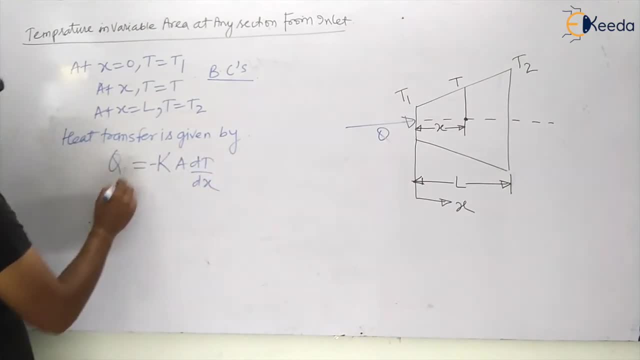 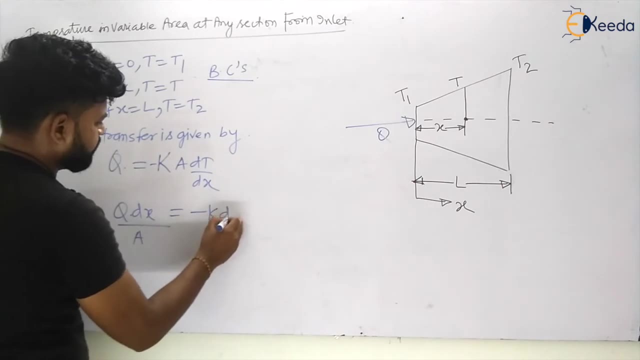 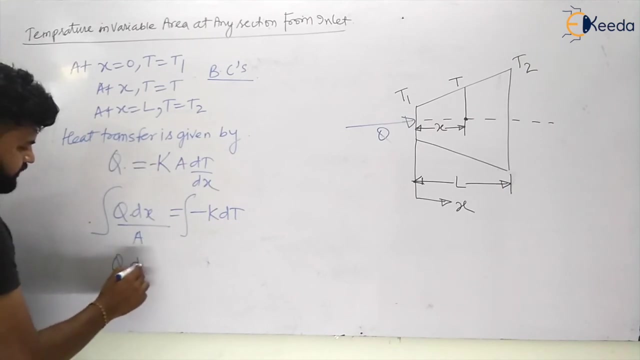 dt by dx. So again, I will take dx this side and area this side, So this will become equal to minus A into dt. So integrating both equations, I can have the temperature That is given by Q into dx by A. 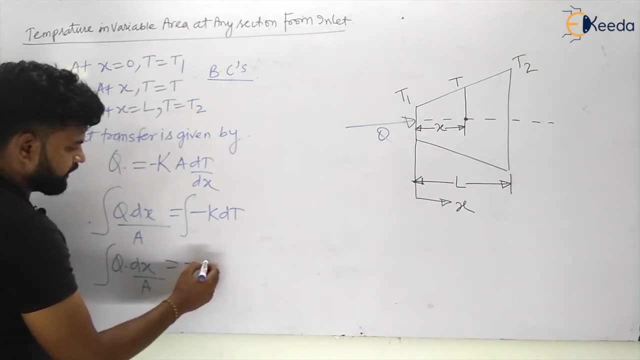 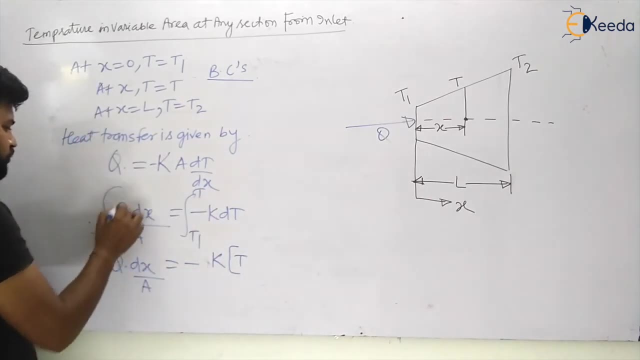 Integration is equal to minus. This will become k and this will become k of that will be t1 to t2.. t1 to t, that will be 0 to x to t minus t1.. So you can, by integrating this equation, 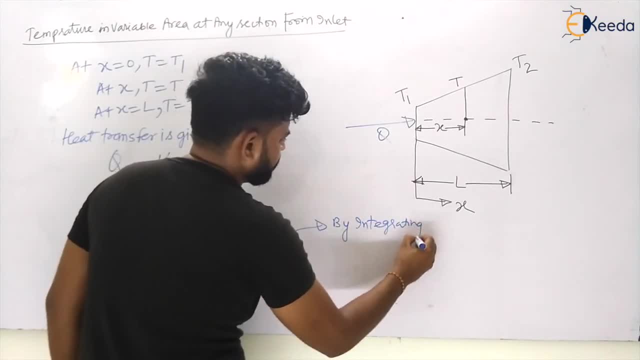 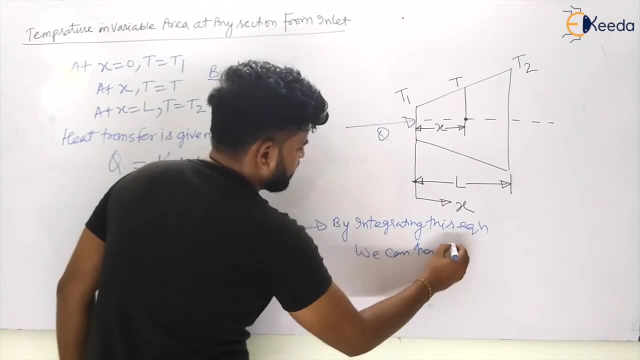 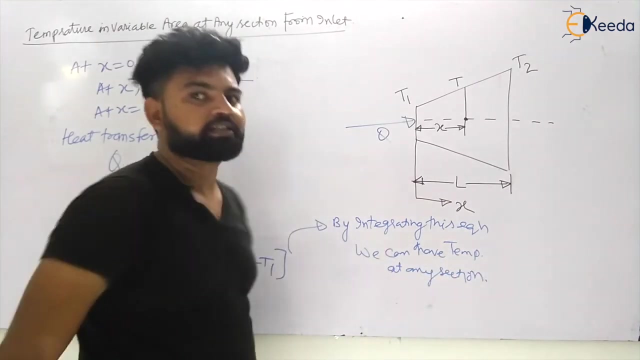 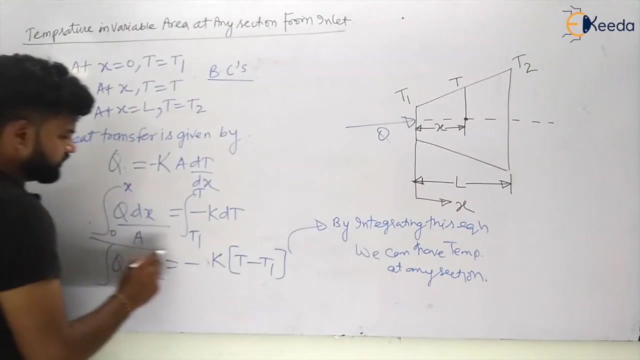 integrating this equation. we can have temperature at any section. I think the fundamental is clear, Clear. my dear students, I can do this, but we will be doing this all in the numericals, So you can easily do this, So you can easily calculate. 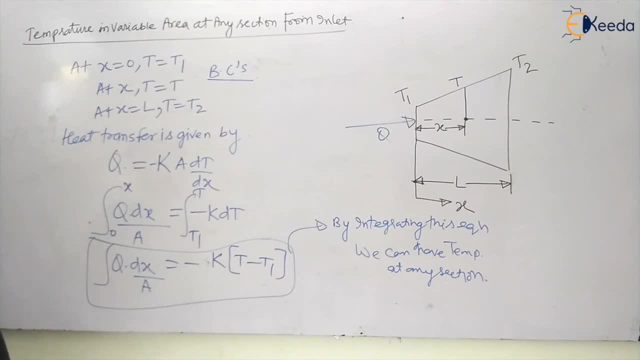 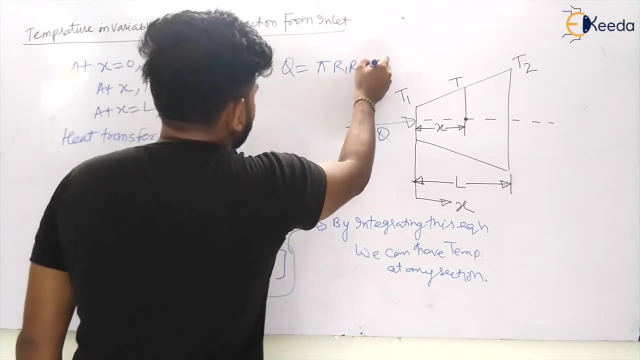 the temperature at any section or from direct formula. also, you can calculate the temperature at any section. What was the formula for heat transfer? It was pi, r1, r2 into k, that was t1 minus t2.. So if you want to calculate t1,. 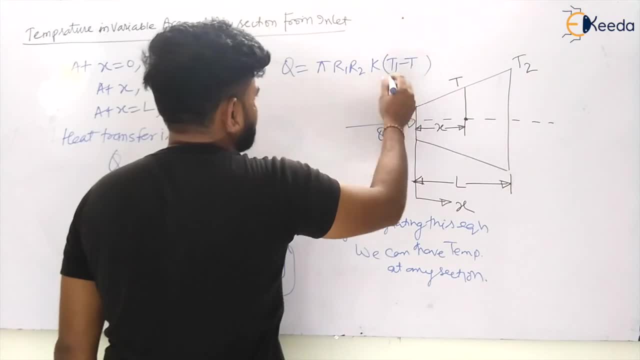 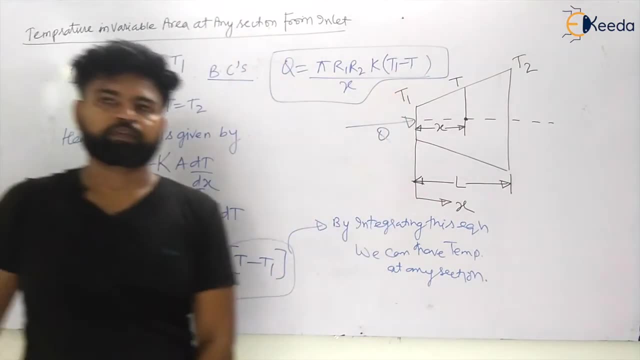 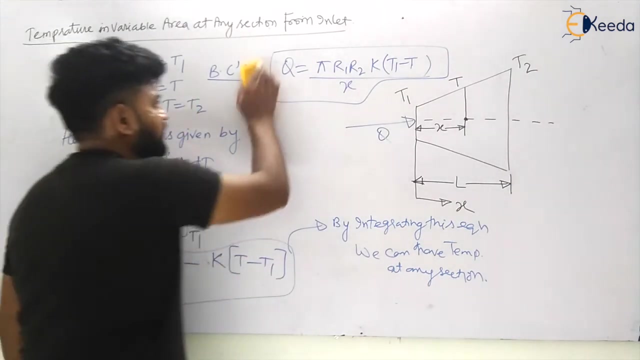 you know. So if you want to calculate t2 at x, so take x down. like this, You can have the temperature directly, Yes or no? You can have the temperature directly. So this was up to it in the variable area. 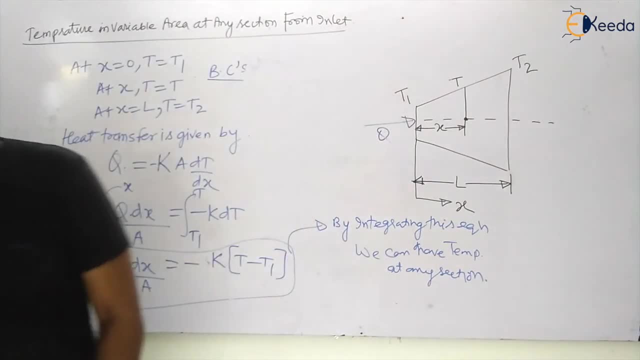 Hope you have understood all the concepts and everything is clear. 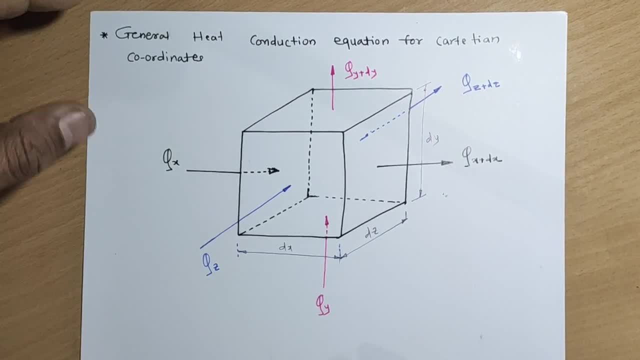 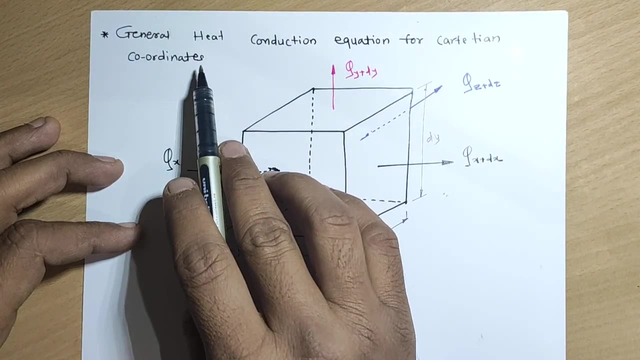 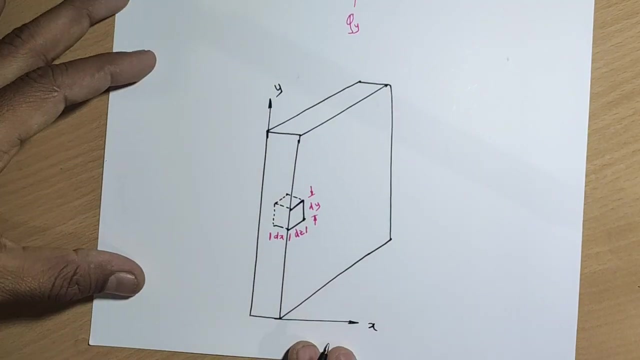 Hello friends, welcome back to my new lecture Today. in this lecture we are going to derive general heat conduction equation for Cartesian coordinate. For this particular derivation, let's consider a figure given here. Let's consider a broad figure. first of all, This is the wall.